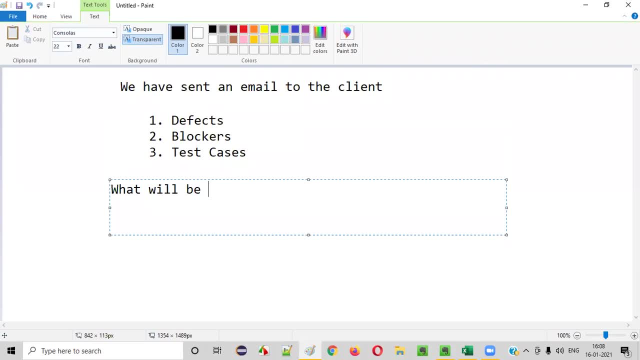 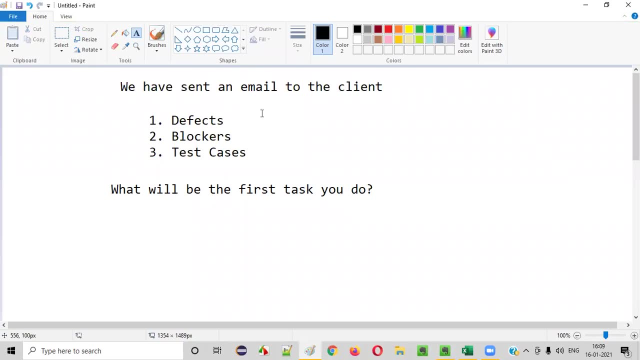 the office. So what will be the first task you do after reaching the office? Okay, you send this email guys to the client and, uh, you came back. so what should be your first task after you reach the office the next day? simple guys just need to check. everyone has to check their email email box because this: 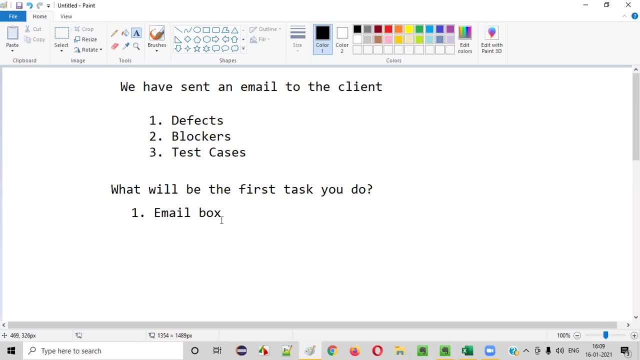 is the place where the general communication will go on, right, so client may have replied to this email. why the client will reply? guys, because you mentioned some blockers. right, the client may have to respond. have a client may have to give some reasons why these are blockers. okay, uh, you can. 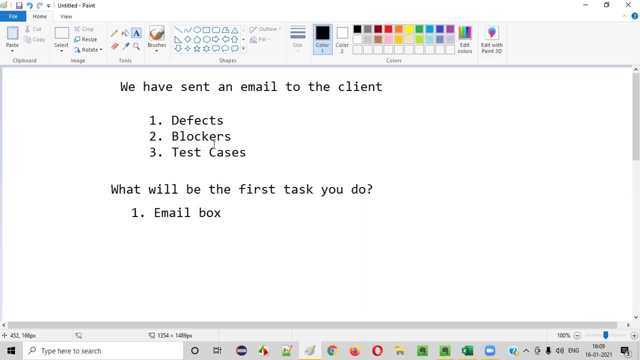 yeah, like you can wait for some more versions or something, something the client has to say in the reply right, it's our duty to let the client know that there are some blockers which we are unable to test right. at same time, client has to reply you with the proper reasons of these blockers. 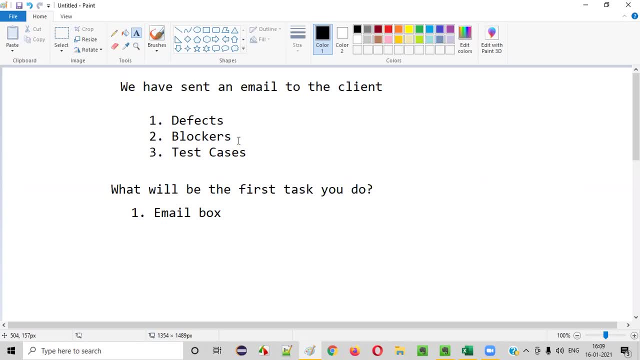 sometimes the client may also give you some uh test data also. for example: uh, there were some situations for the blocker test, blocking test cases, right, the coupon codes were not there, right? uh, how to check the coupon code functionality if you have the coupon code only? coupon code only. you can check the coupon code functionality if you have the coupon code only. 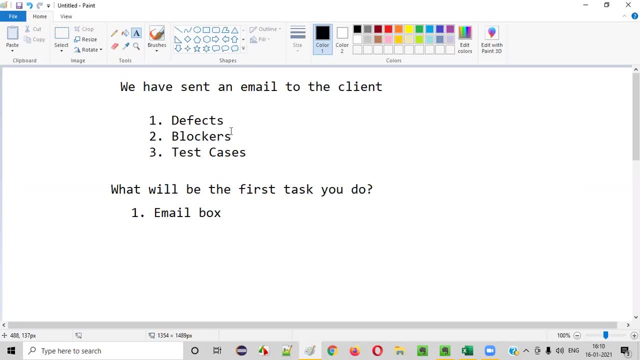 then you can check. the client may generate such kind of coupon codes for you and i may put that in an email and send it to you for your testing purpose. like that many emails you may get from the client, guys, because of the previous email that you have sent to the client, and, uh, next thing is: 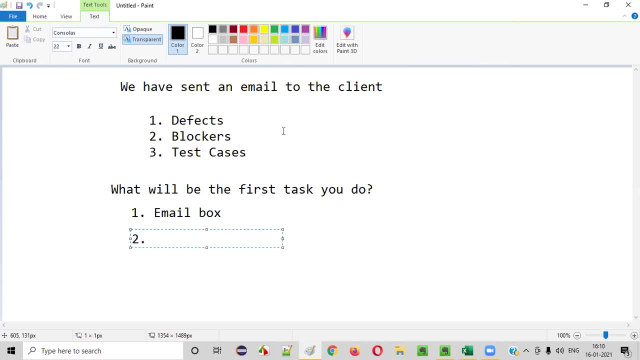 next thing after checking the emails. okay, let's say, you got the email and, uh, you understood whatever it is in the emails and that's fine. okay, next thing is. next thing that it has said this is he will open the bug tracking tool. okay, after checking the email. 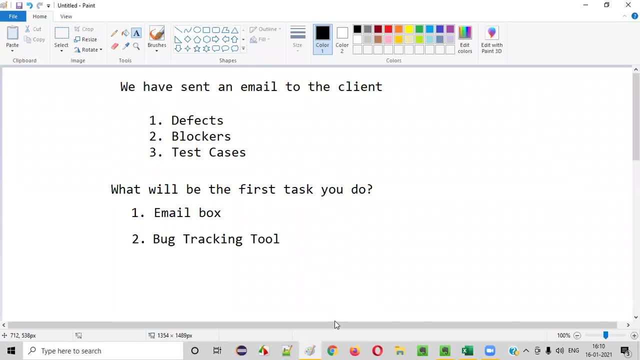 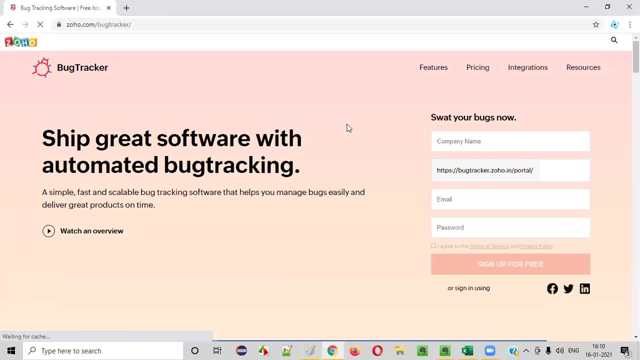 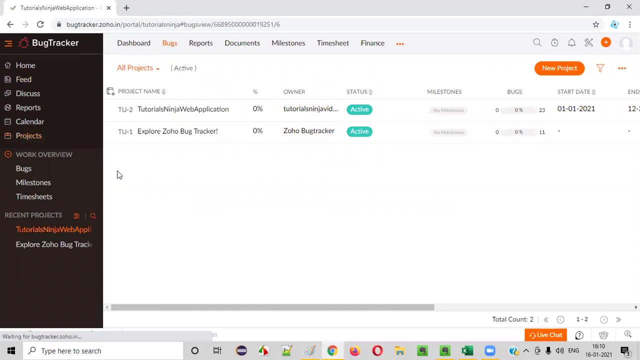 bug tracking tool is the next thing. okay, so let's open the bug tracking tool. we were using the ZOHO bug tracker as a tool for uh reporting our defects. right, this is provided by the client, assumingly. now open this. go to the project that you are working, select the project and you can see all. 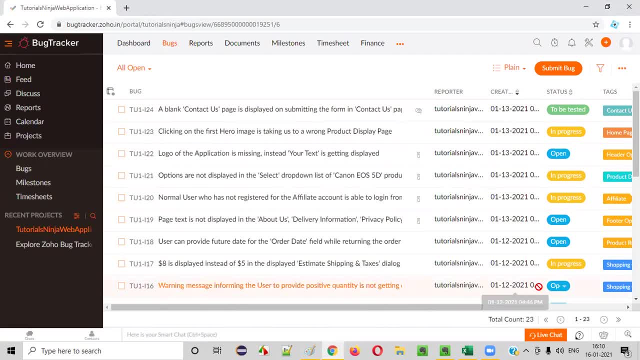 the list of defects that we have reported earlier, right, the past few days. whatever the defects we reported are displayed here. but, guys, when we report the defects, by default, the defects will be in open, in open state. right, whenever we report the defects by default, they will be open state. 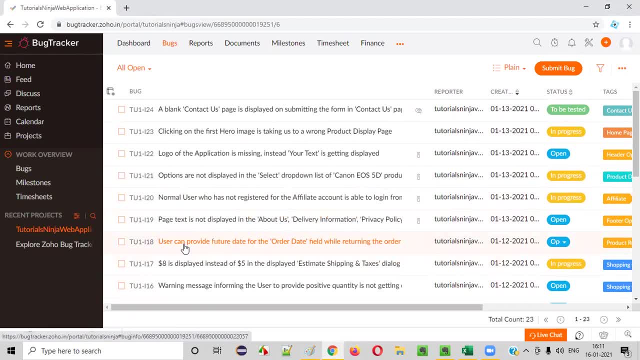 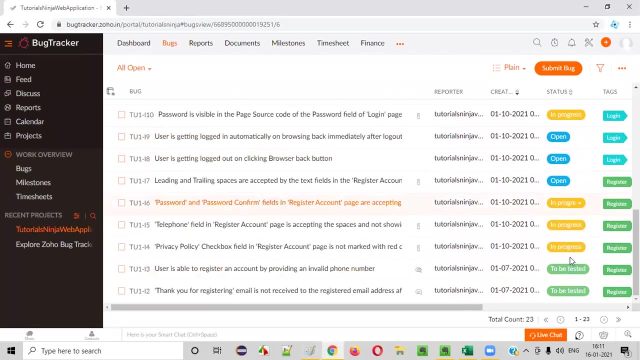 but when a developer starts working, okay, when the developer starts fixing that particular defect in this particular zoho bug tracking tool, the status will be changed to in progress. okay, developer will change the status to in progress and then he will start working on this particular defects. okay, whatever the defects that you are seeing here on this list of defects which. 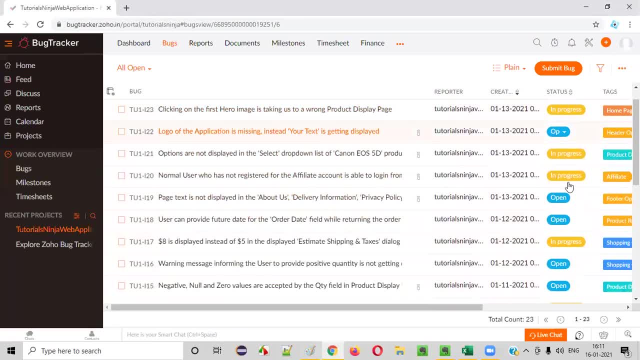 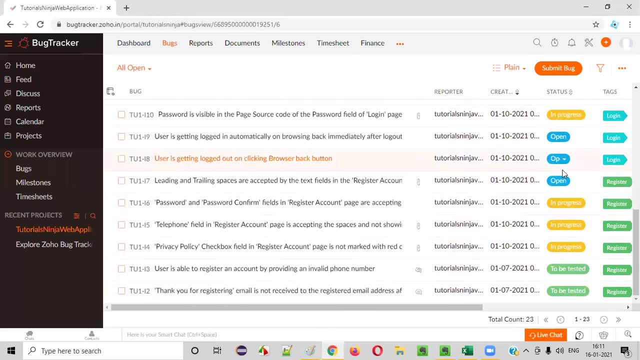 are in progress means the developers have started working on this particular defects. fine, simple. now, apart from this open and in progress, there is one more status also being displayed, guys, that is to be tested here. here also, some two defects are in to be tested here. one defect is: 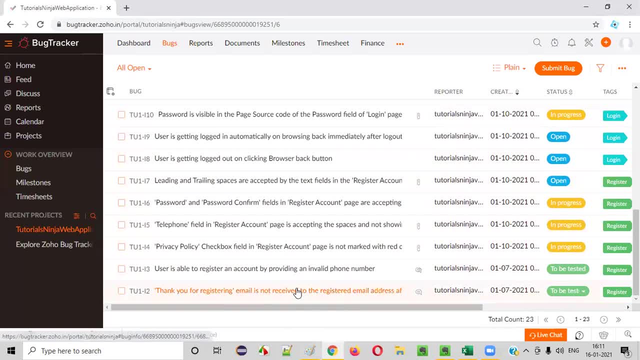 also in to be tested. total three defects are in to be tested. to be tested means what to be tested means this: this status is also changed by the developer guys. initially, few defects were changed to in progress and now developer have completed fixing this particular defects. okay, while in progress, the developers have 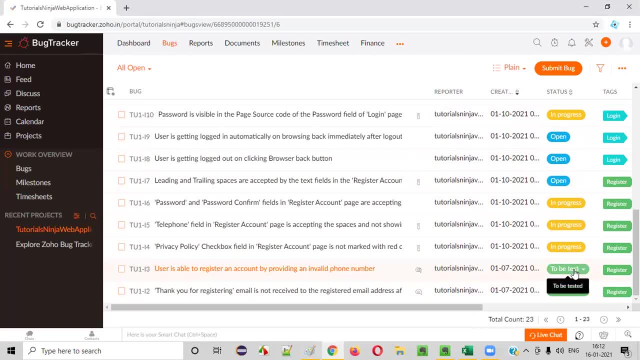 fixed the defects and then he changed the status he or she has. he or she- developer- have changed the status to to be tested. that means the fixing of this particular defect is completed. now it's your turn. as a tester, you need to test it. so that is that is the thing, guys. okay, to be tested, fixed. 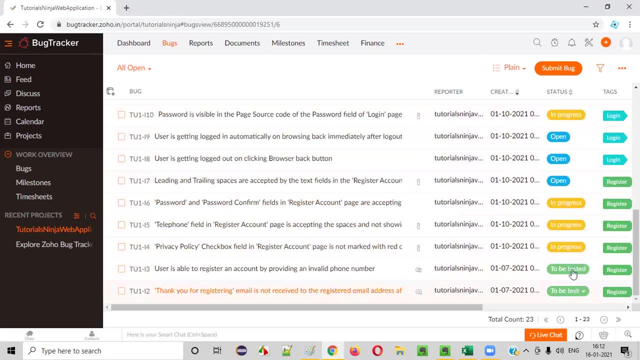 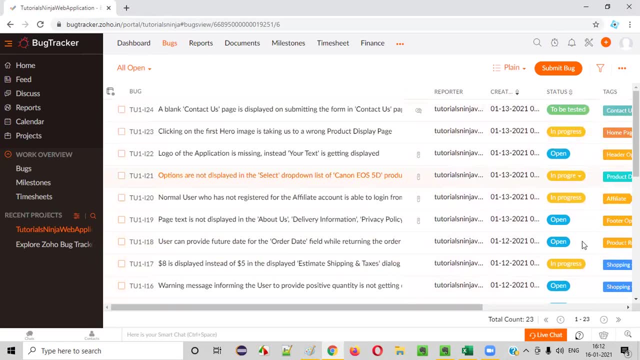 or to be tested. both are same. in zoho bug tracking tool it's called as to be tested, fine, to be tested. so when you are testing a particular defect, the developer is going to do a test right after the. you receive this to be tested right in progress. open and in progress doesn't matter, guys, because 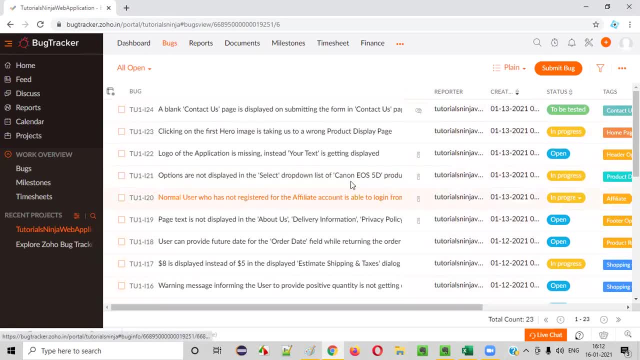 in progress are still being worked by the developers right, while the defects are not fixed completely. you cannot test them right, these defects. you cannot recheck them. so only the things that you can take from here is that uh to be, uh to be tested. that means the fixed defects case. 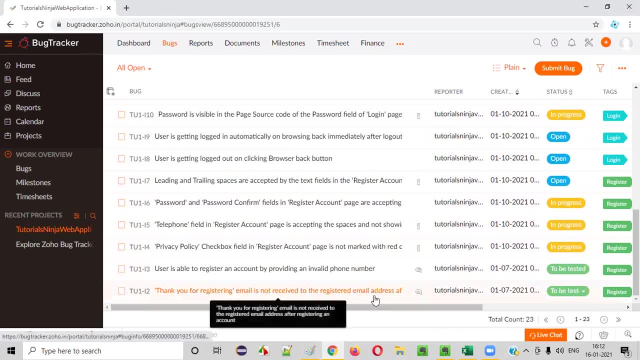 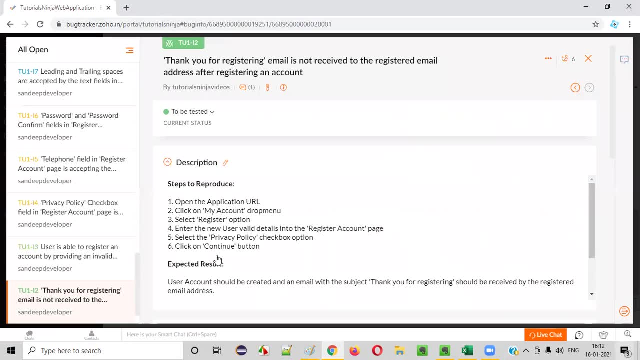 to be tested means fixed effects. let's go with the one on one, one by one defect which are in to be tested state. that means fixed state. so let's open this. uh, yeah, this was a defect, guys, and when you scroll down somewhere here, developer has put a comment saying that: fix it in this. 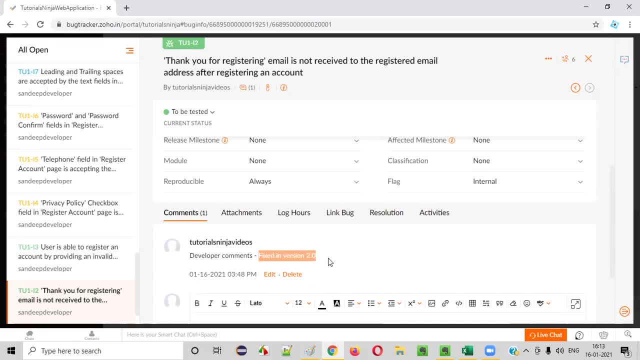 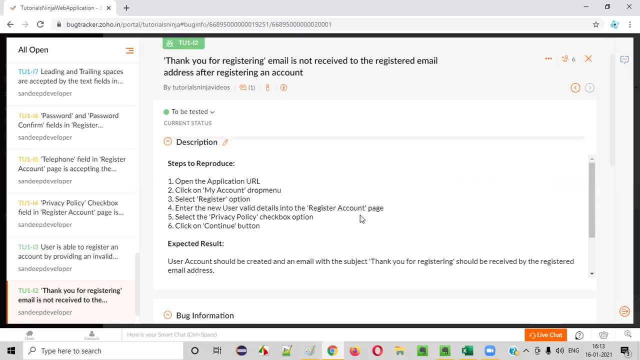 version 2.0. okay, the version of the application that we have tested while reporting this defect was 1.0, let's say. now developers have started fixing the defects. they have really fixed it and changed the status of the defect to be tested, and they have added a comment here. 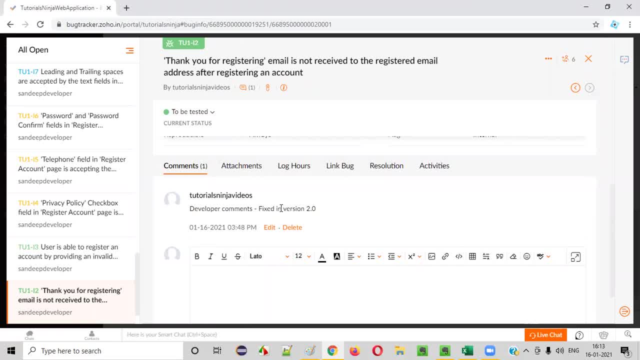 saying that, saying that the defect got fixed in the version 2.0, guys, okay, another version of the application will be given. okay, whatever the version on which the developers have fixed the defect, right that that application will be given for us for our testing. okay, we should not be testing, uh, this defect again on the same. 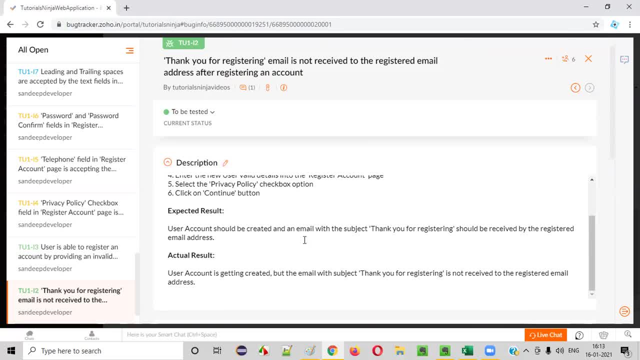 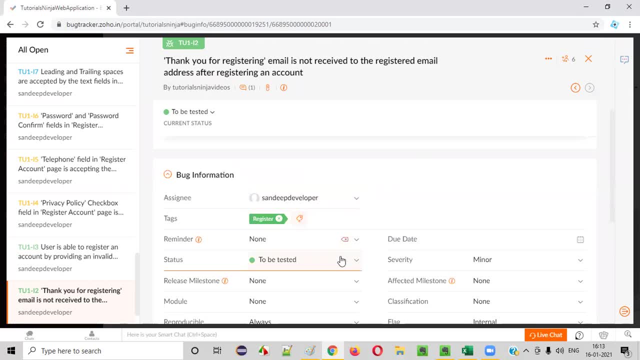 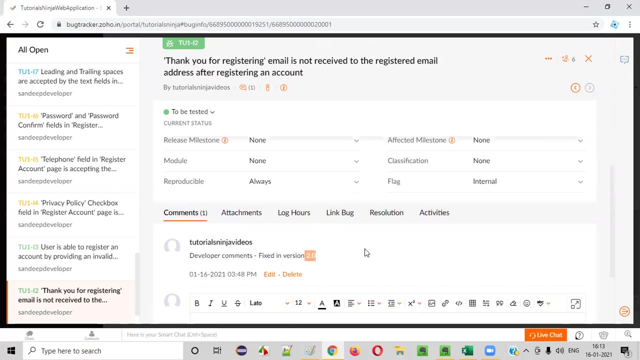 version that we are testing. okay, so developers have fixed this defect on the latest version of the application. we need to wait for this particular application. then only we can retest these defects, assuming that, assuming that we got an email from the client with this version 2.0 of the application. 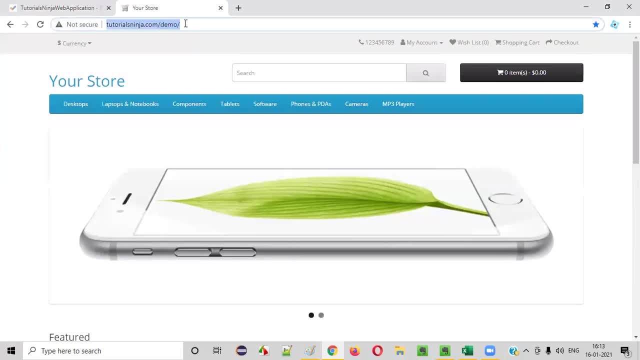 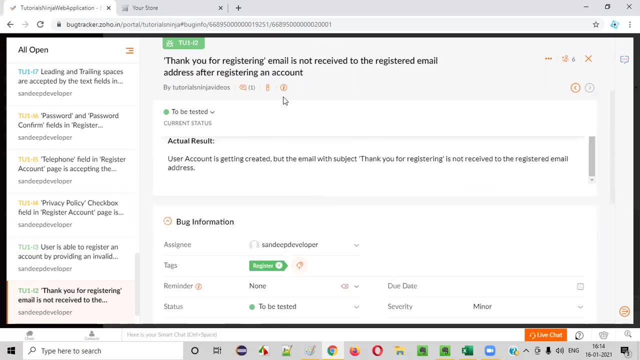 okay, let's say this is the same. same same version again. okay, same application again. so this is a 2.0 version, assuming that and developers have also mentioned that this particular defect got fixed in this particular application version 2.0. okay, let's say this is a. 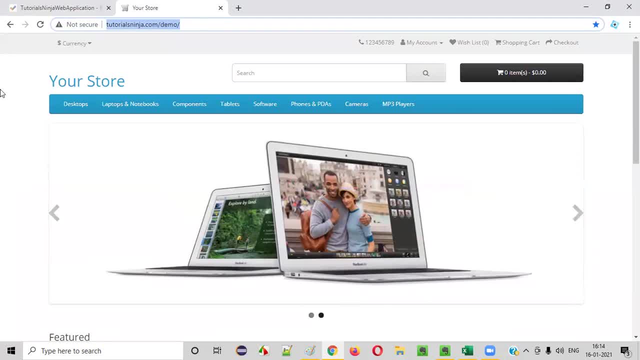 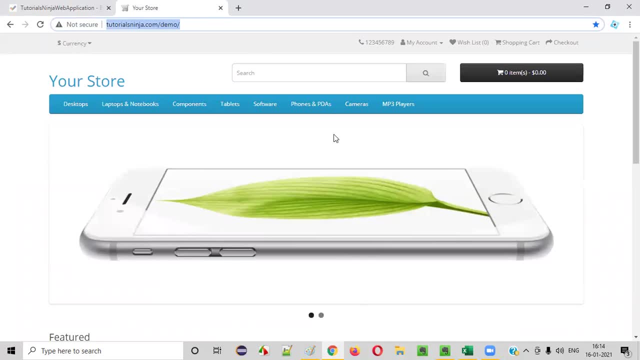 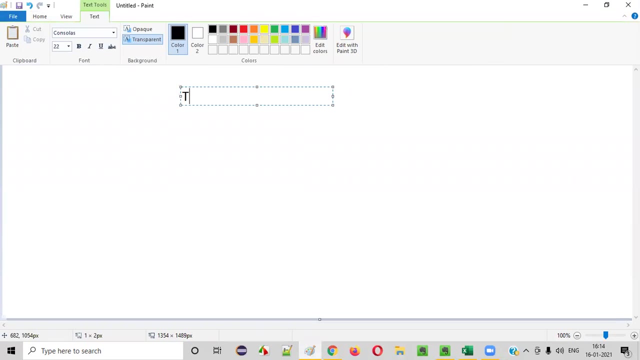 2.0 version. only now, guys, what you will do. so the first thing that a developer tester has to do, after he received this kind of things and the appropriate version of the application right in which this particular defect got fixed, he will do the next thing as retesting guys, he will start. 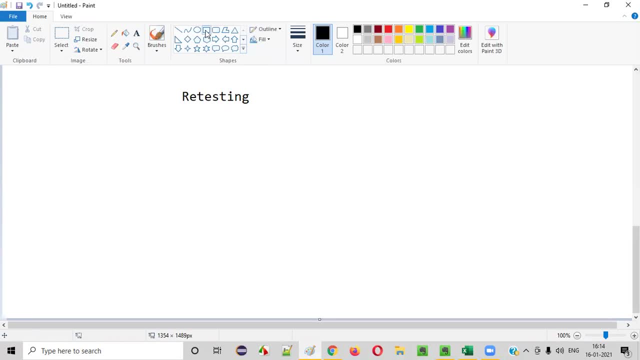 retesting. what is retesting, then? what we have to do, what the software tester has to do as part of retesting, once we receive the fixed defects, along with the version of the application in which the particular defects got fixed. okay, these two things you have to remember. okay, once you receive the 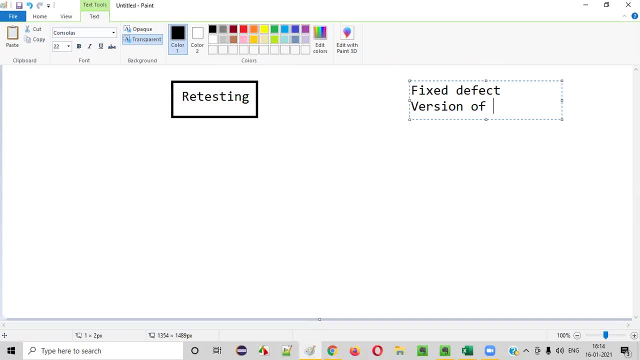 fixed defects and you get the version of the application in which the defects got fixed. got fixed. okay, these two things. if you get fixed defects but you didn't get the version of the application in which the defects got fixed, then you can't retest. right, both should be there. these two things should come first of all. 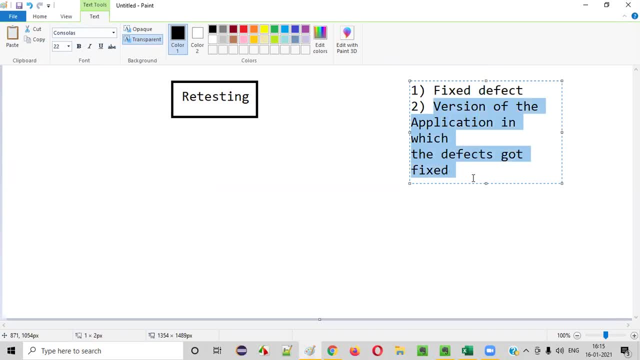 the defects should be fixed and also you should get the version of the application, the latest version of the application in which this particular defects got fixed. okay, all these things here, all these two things you need to get. once you get this version of the application, you can retest. 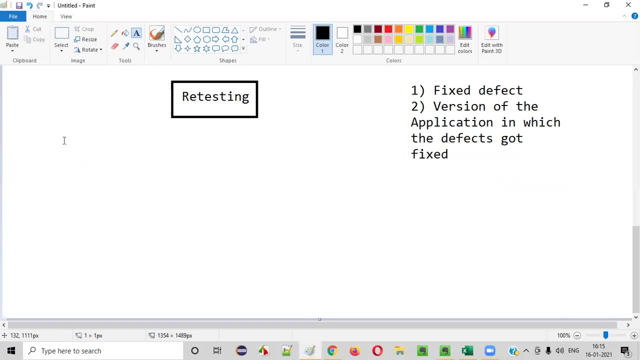 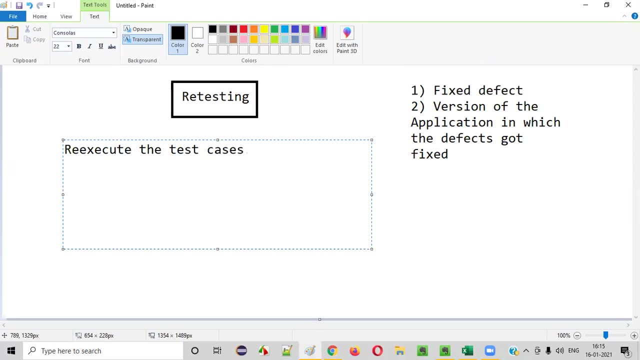 these two things, then you will start retesting guys. so what you will do as part of retesting? we have to re-execute the test cases- okay, related to this failing. okay, related to this, defects which got fixed. simple, we need to re-execute the test cases related to the defects which got fixed. so 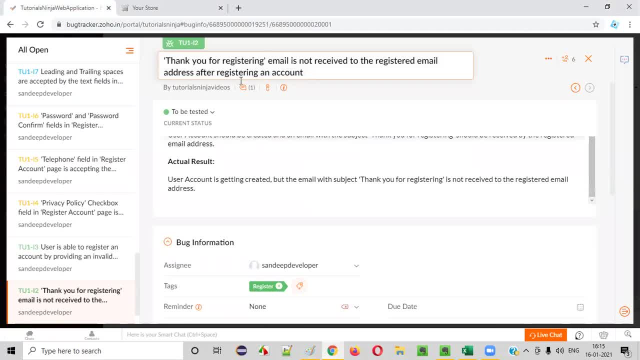 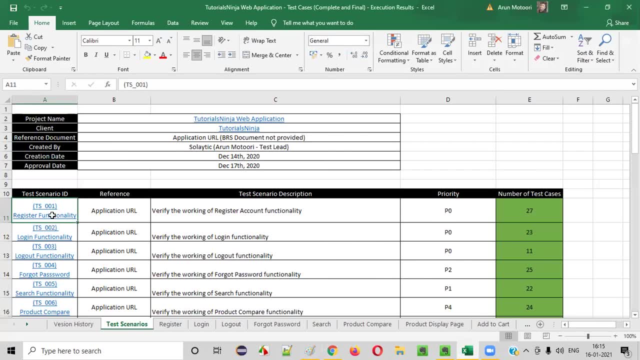 let's say, uh, what are the defects that got fixed, guys. one of the defect was: uh reached string email. right, it belongs to the register functionality. let's uh go to the test case document. so, register functionality. let's go to the particular test case, uh, for which? okay, these are: 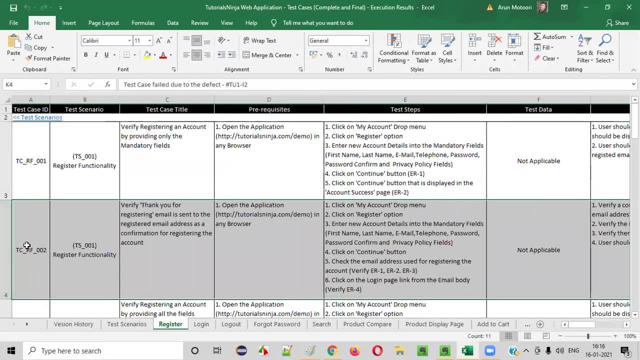 this is the one right. this is the test case. this is the test case, guys. thank you for registering. email is sent to the register email address as a confirmation for registering the account for this particular test case. we have reported this defect. now the developers have fixed this defect okay. 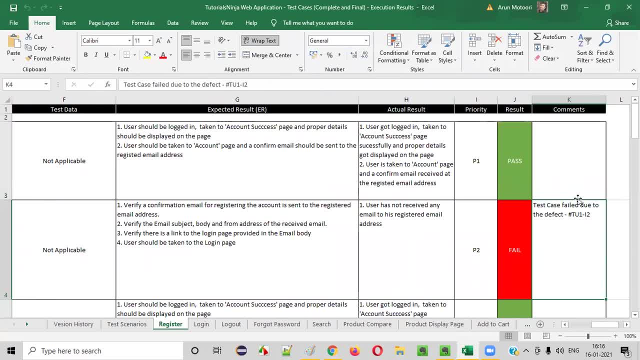 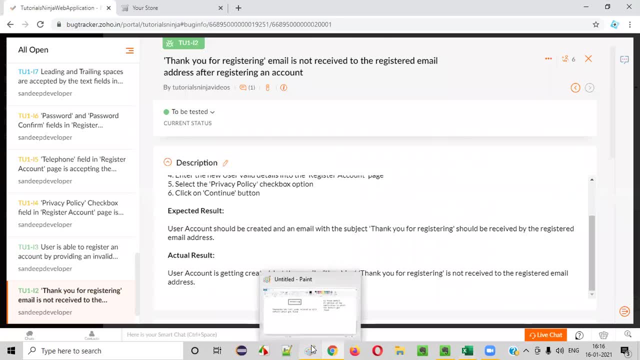 tu1, hyphen i2. okay, let's say, the developers have fixed this particular defect and, uh, we were asked to, we'll be performing the retesting in simple terms. okay, so as part of retesting guys, whatever the test cases that are related to this particular uh fixed defect, that is, uh, the test cases related. 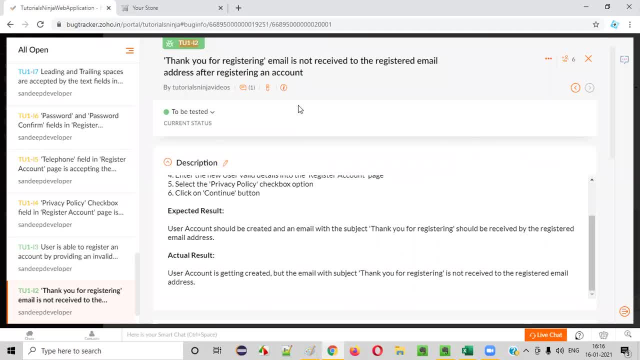 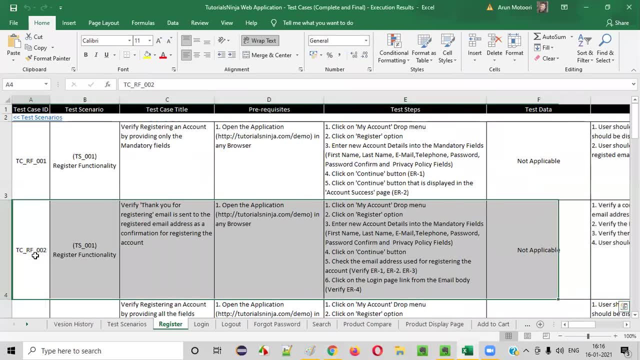 to this: tu1 hyphen i2 need to be tested. so we'll open that excel like test cases document and we'll execute this, re-execute this particular test case. okay, let's say, after you re-executed this particular test case as part of retesting. 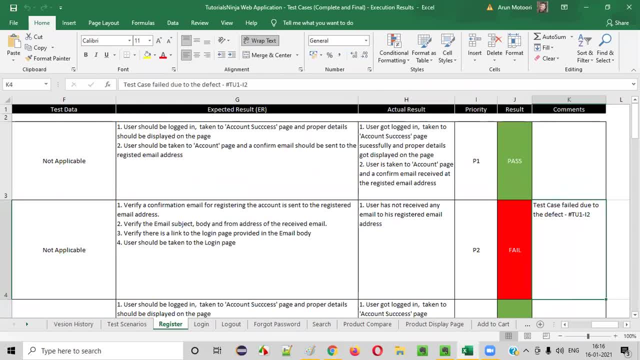 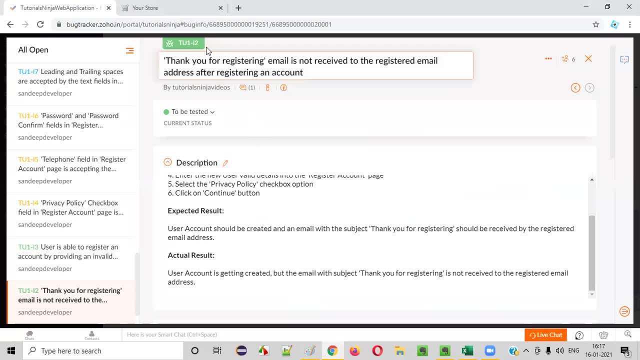 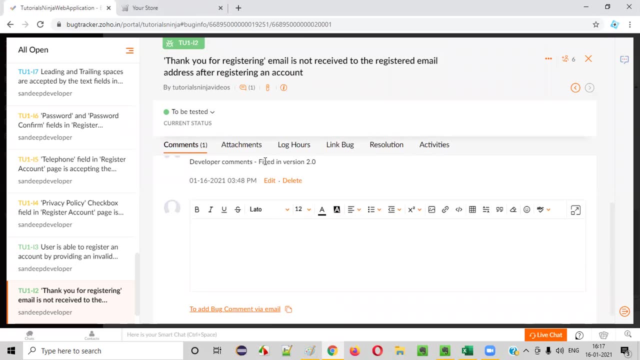 you are retesting this particular test case of this particular fixed defect. now you got the result, as still you are not getting the emails, even after, even after the developer have fixed this defect, even after the developer have mentioned that this defect got fixed in this particular version 2.0, and again when you test the same test case. okay, we need. 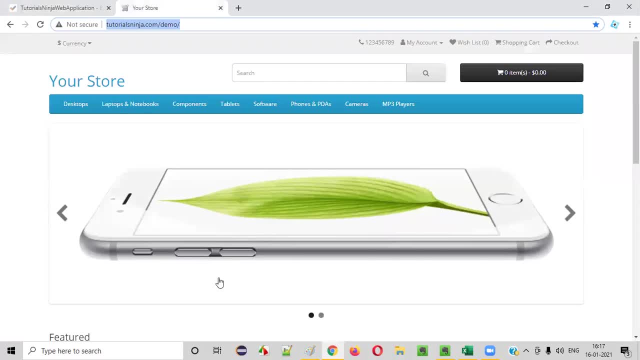 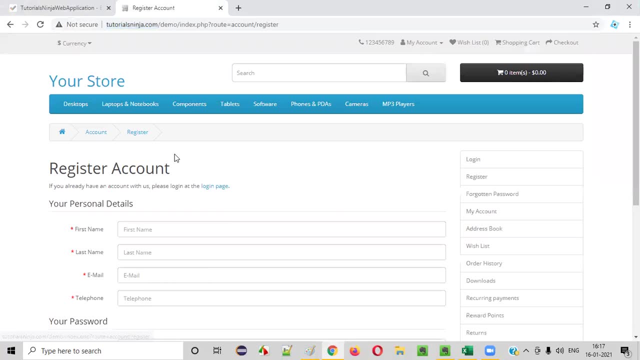 to follow the steps again, guys. okay, again, we need to open the application like this: and then this is a version 2.0 in which the defects got fixed. and then we need to click on the my account drop menu, click on the register. you need to provide the details, okay, uh, let's say: 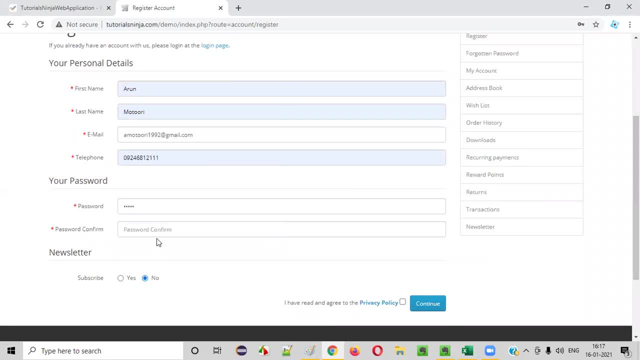 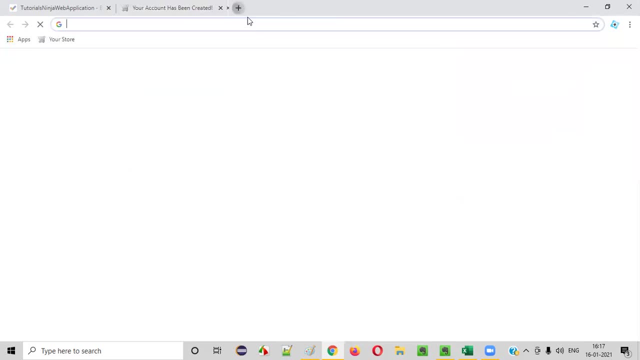 okay, something, uh, one. okay, some password and then continue. okay, account is created. now again, if you go to your, these are the steps, right, we have to follow. you have to enter all the details, click on continue button. we need to check the email address. okay, whatever the registered email address i give and write a motor amotory1992.gmailcom. so we need. 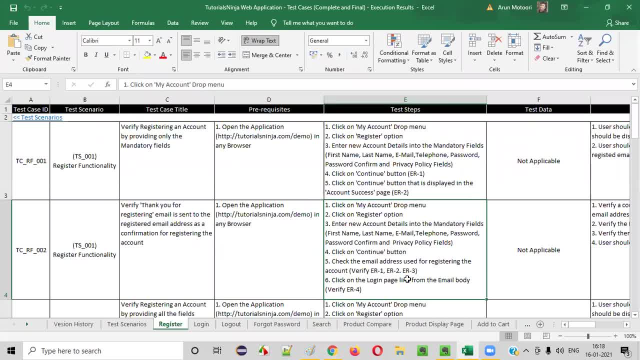 to go to that email address and see whether we have received any email from the application as part of welcome email kind of thing. thank you email kind of thing. did you get any? thank you for receiving email, let's say, even after creating this account on the latest version of the. 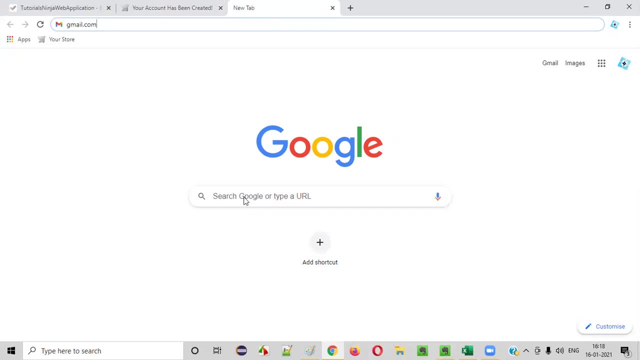 application where the device got fixed. still, if you are not receiving any email to your listed email address, what you will do? guys, this was a failed test case. right, it was failed. now the developers have mentioned that it got it's ready for testing, but when you retested it, 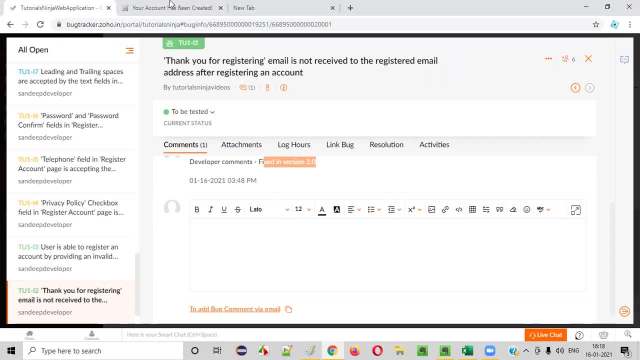 on the latest version, in which this particular defect got fixed by executing this particular test case again. what happened was: this defect is still reproducing for you. okay, as a tester, you are able to replicate the defect in the latest version also. so what you will do here is you will change the status again, guys. okay, you will change the status. 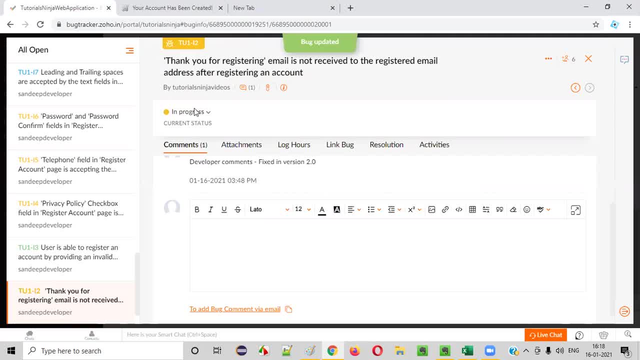 again to in progress. okay, you need to assign it back to the developers. here you will write the comments assigning it back to the okay developers, as the defect is still reproducing in the latest version of the application. that is what is the latest version. that is, application version 2.0. whatever the version, 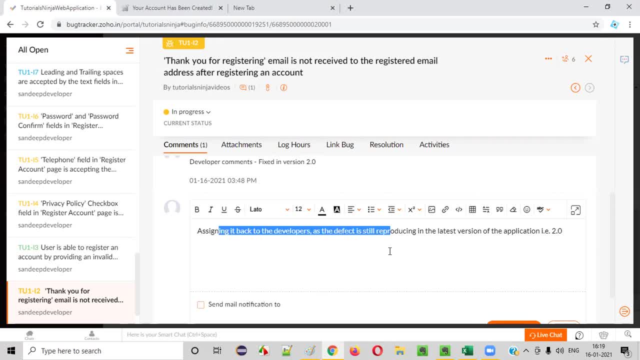 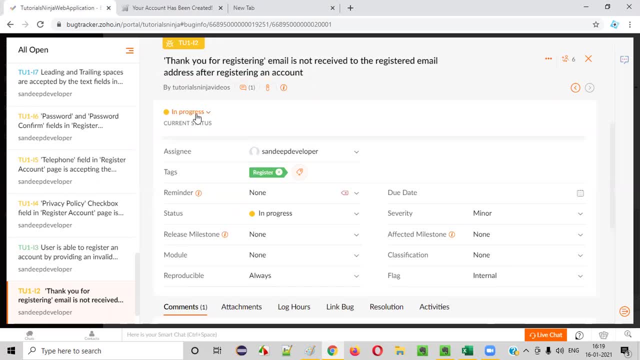 the developer have said that it's fixed. it's not fixed for you right when you retested it. unfortunately, the defect is still reproducing in the latest version also, so you have to change it back to the in progress, where developers have to work, and then click on add comment. so this comment will be added. that's it, developer will. 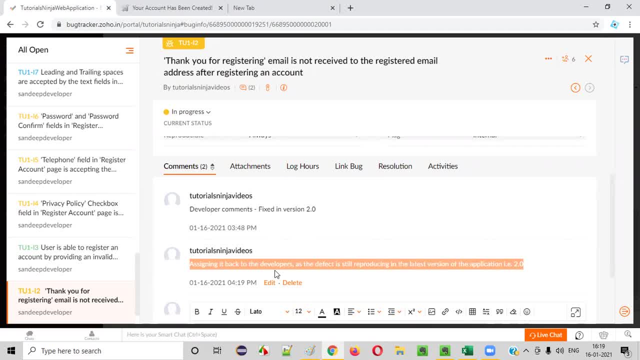 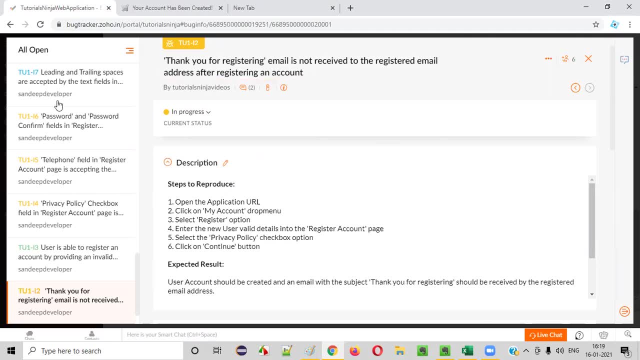 receive a notification in his email box with this particular comment so that he'll look and start working again. okay, and you will try to fix that in the other version of the application, the next latest version of the application you try to fix. so this thing happened and, uh, you will not change. 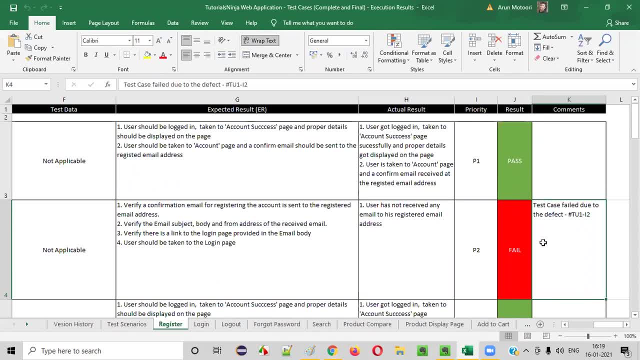 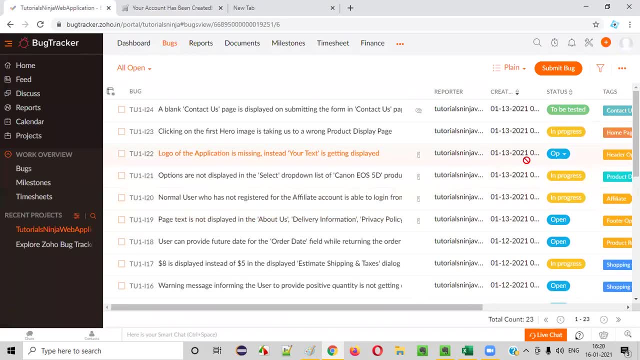 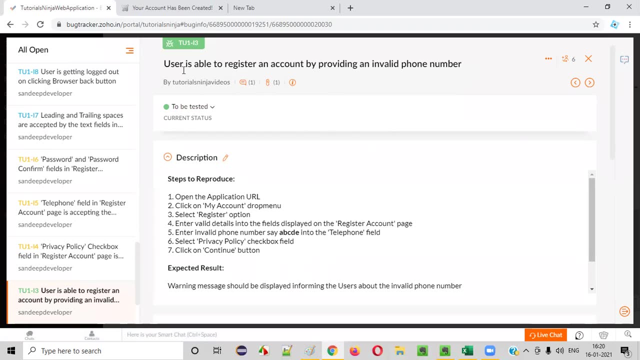 this particular fail. okay, you will keep this failure as as it is because, you know right, you tested in the latest version and still it's failing. fine, so this one again changer to in progress. then what about the another one? okay, let's say you, we will take another defect, which? 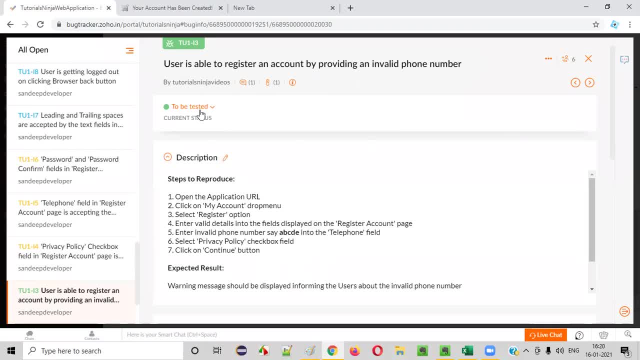 got also fixed. okay to be tested state is there. that means it got fixed. now, tester as a tester, we need to retest it. how to perform retesting of this particular defect? this particular test case is related to which functionality? guys register functionality only. let's go to the particular test case for. 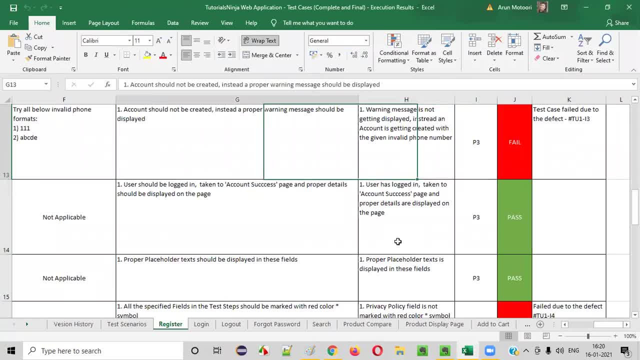 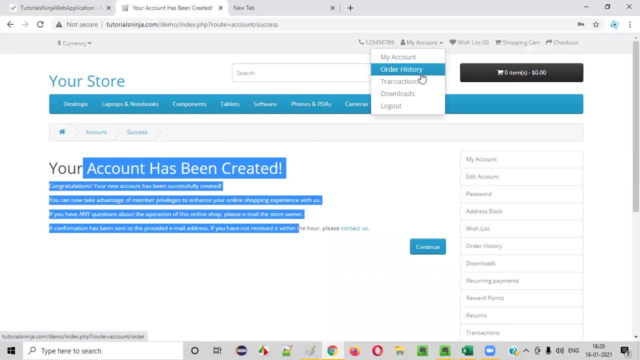 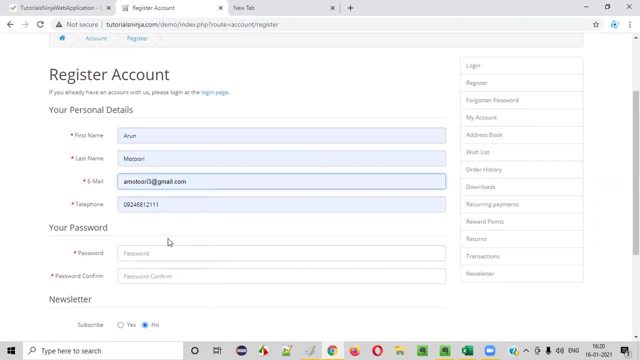 which this defect was reported. so this was a defect. okay, so verify registering an account by providing an invalid phone number. when you try to create, okay, when you try to register an account by providing an invalid phone number, okay, okay something. and here let's say, let's say: 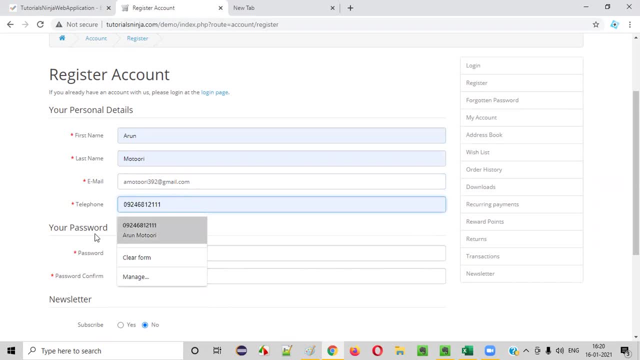 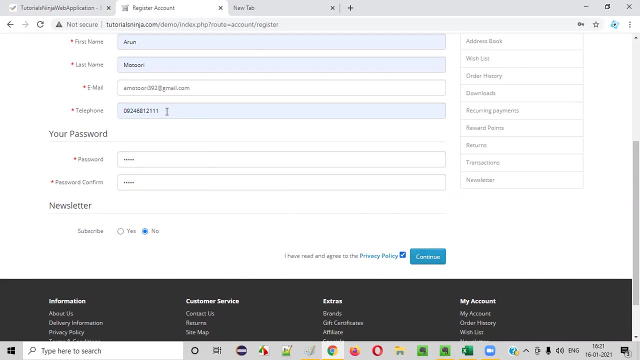 this is an invalid phone number for now. okay, let's say this is an invalid phone number and when you're trying to create when, when you're trying to create an account with the invalid phone number, this is not invalid, guys, but let's assume that this is invalid, okay, and 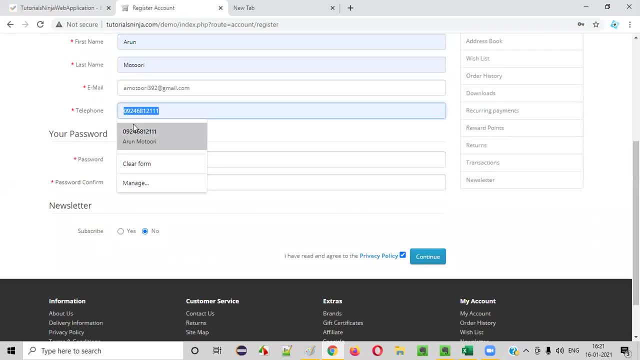 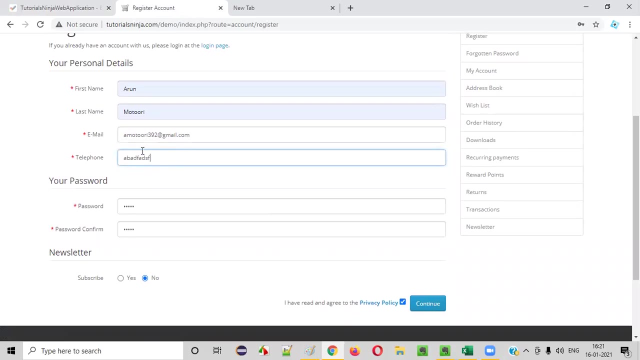 uh. so let's say this is invalid, right, okay. so something okay like this is invalid. now, when you click on continue, let's say you are getting a field level validation. now assume that okay, because i cannot fix this application, guys, so just assume that this time, when i gave the invalid phone number here, like abcd or something, 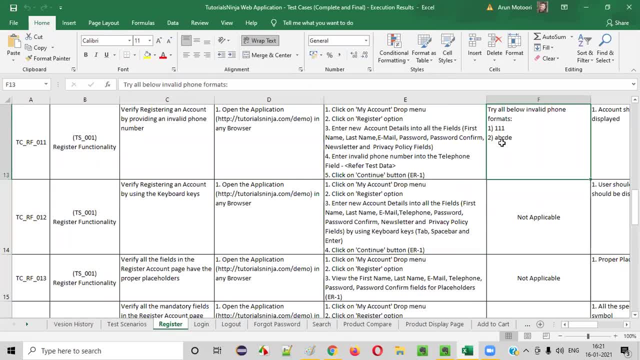 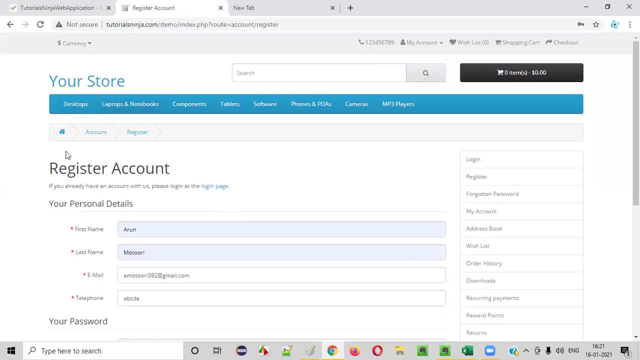 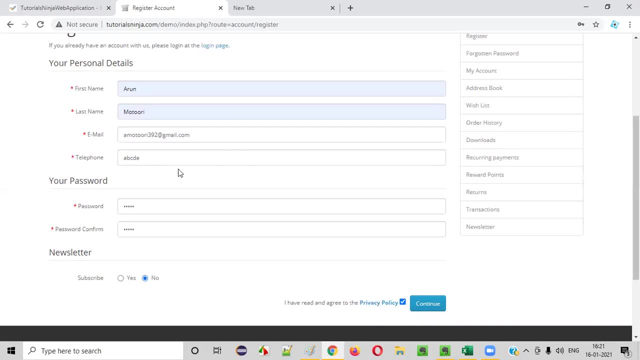 as per the test case, i have to give some invalid phone number like abcde. so let's say i gave ab, c, d, e and then when i try to click on, continue, guys, i got a warning message here under the telephone saying that enter proper telephone number, okay, or like proper telephone format. 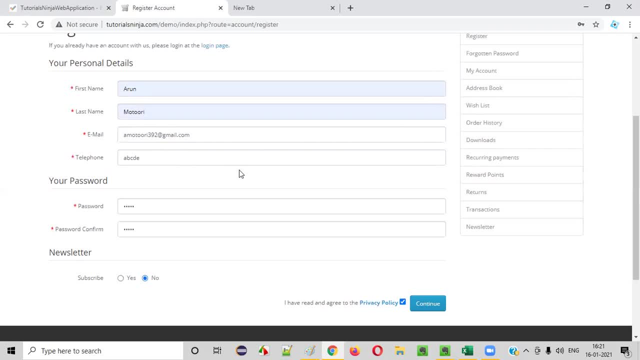 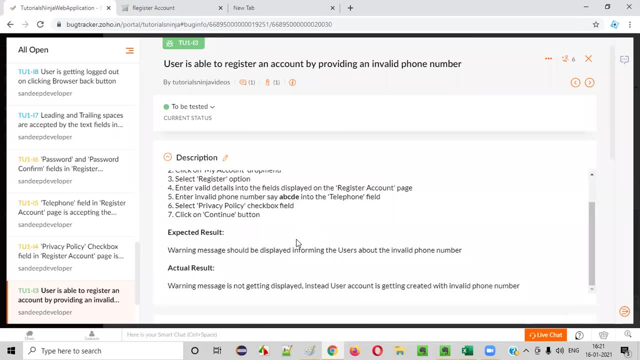 need to be entered. whatever the kind of warning message that got displayed, assume that okay. let's say that is getting displayed. now that means developers have successfully fixed this particular defect. so what you will do in that case if the this particular defect is not reproducing in the 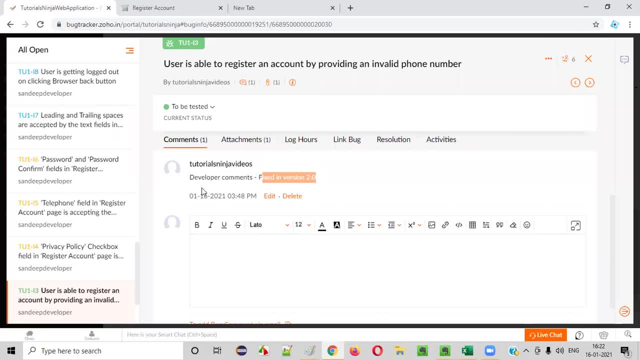 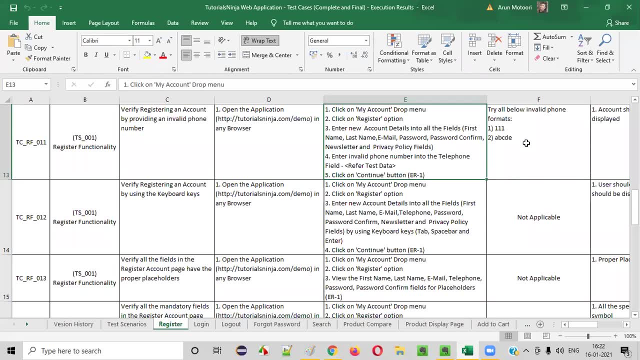 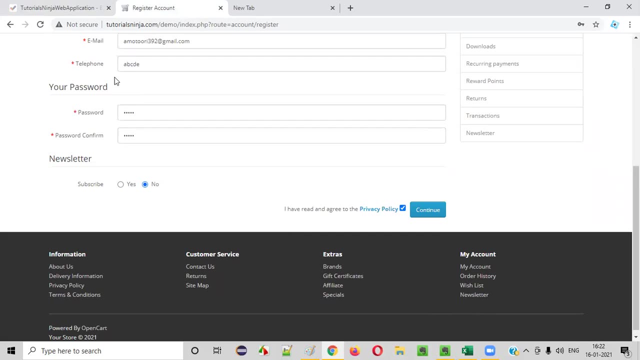 here. you see, the developers have changed the status to be tested and they mentioned a comment saying that fixed in version 2.0 and used you. you actually retested this. okay, you re-executed the test case related to this particular defect and then you observed that the account is not getting created. instead, you are getting a warning. 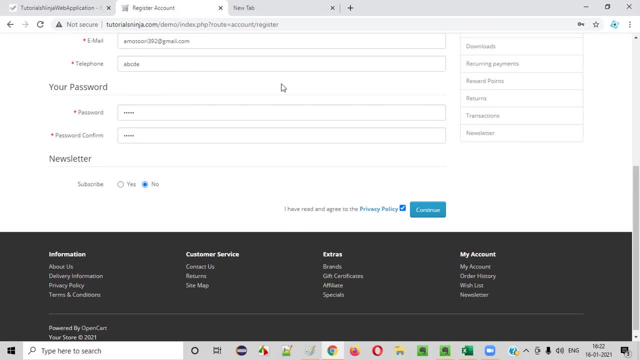 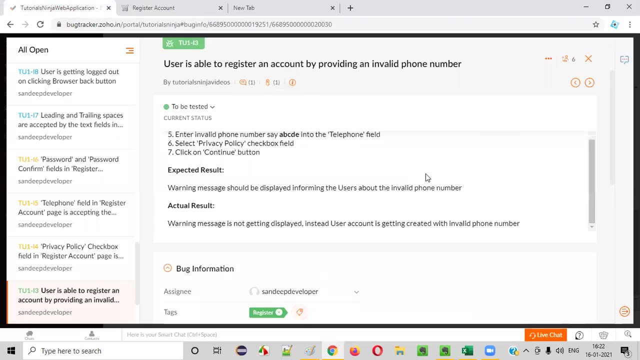 message saying that: uh, invalid phone number is provided. please provide valid phone number. some warning message is coming. so then, then that means that this particular defect is fixed, really right. what you will do at this time is, you will simply, okay, you will put a comment here, guys saying that: 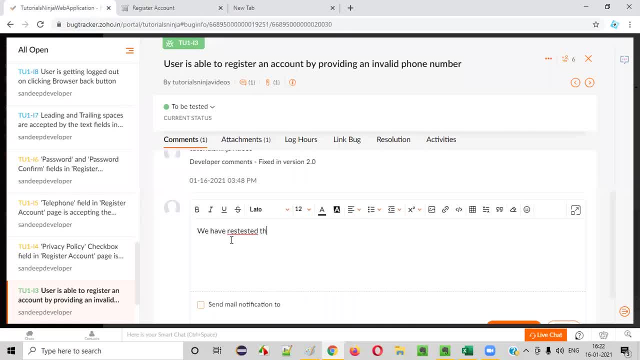 we have, okay, retested this defect in the latest version of the application, that is, 2.0 version. okay, and i have observed that that that it is not reproducing. okay, it's not reproducing. that is, the functionality is now working as expected. okay, now the functionality is working as expected. 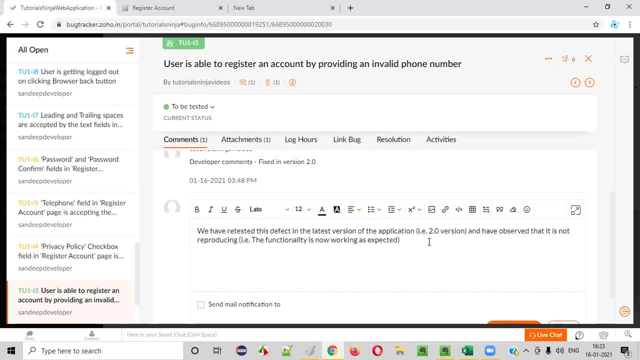 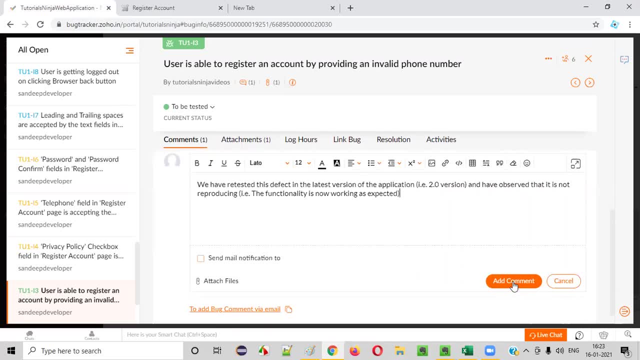 so like this: whatever the way you want to write the comment, you can write, guys. okay, it doesn't mean that you have to write in the same way. i generally write like this, so your way of writing may be different, okay, so up to you. so just add comment and after adding the comment, guys, simply. 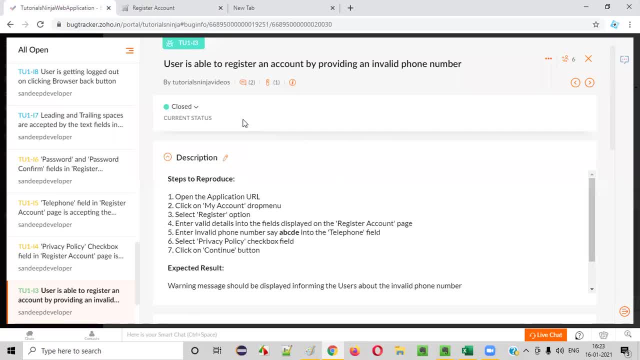 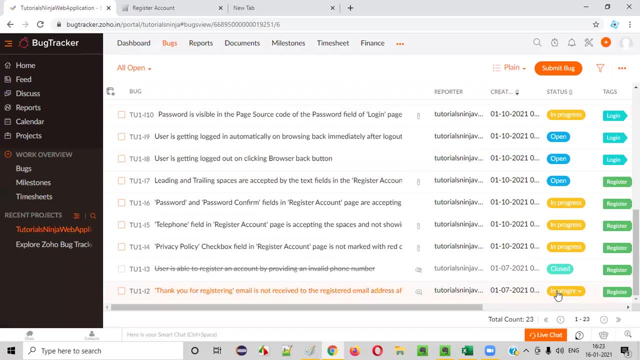 close this defect. simply close means it's done. okay, the defect is properly fixed. that's it, guys. okay, there are two ways right to respond. one thing is like: if the defect is still reproducing for you, you have to assign it back to the developers by changing into in progress and you have to put a comment saying that still, the effect is reproducing. 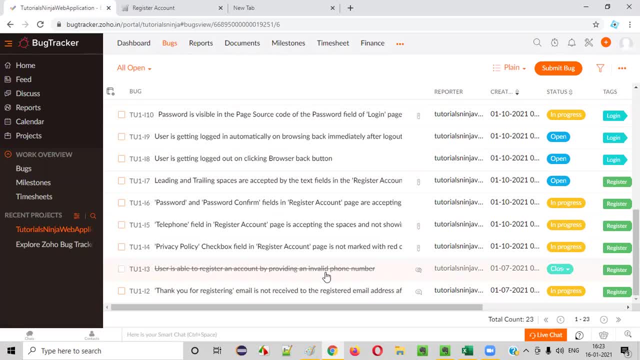 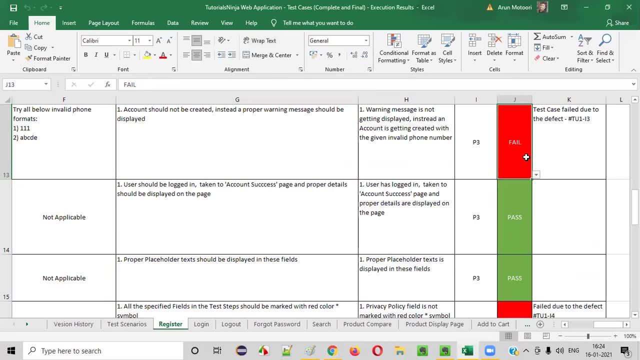 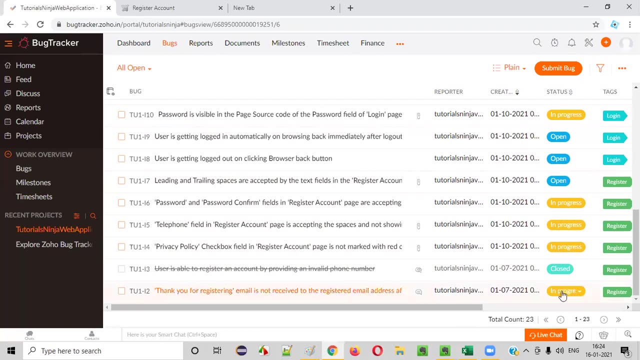 and the other thing is like: okay, other thing is like, if the defect is not reproducing the latest version, you need to close the defect. now, once the defect is closed, guys, you can change the status. guys, okay, so change it to pass and uh, that's it done. okay, that's it so like this, guys. okay, like this, we have to do. 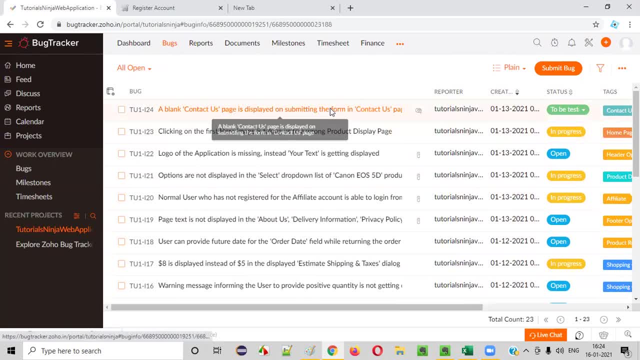 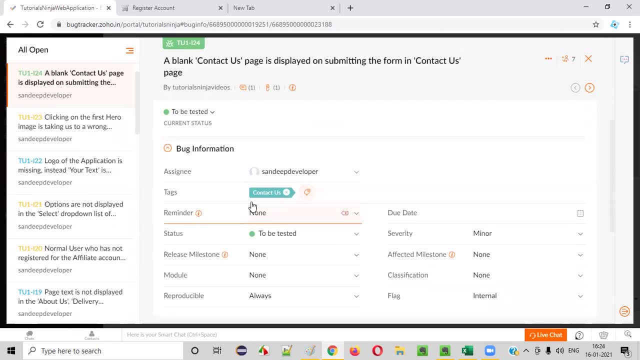 now one more defect is also there to be tested effect. let's say this defect is also still reproducing. okay, so let's retest this particular defect. how to retest this? belongs to which functionality? guys contact us. so let's go to the particular test case, uh, of the contact us. 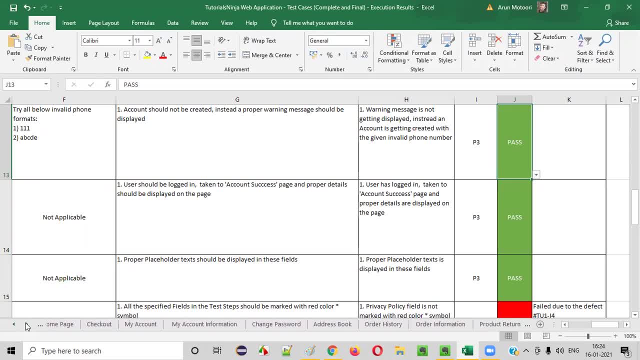 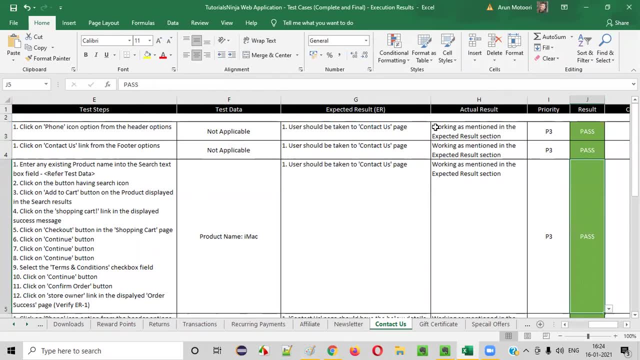 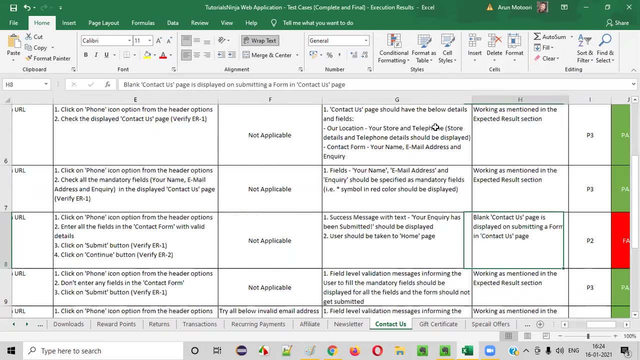 functionality. let's go there, contact us, contact us. so this is the contact us. go to there and find that particular test case for which the defect was reported. is it contact us? okay, what is the defect? id guys, i can compare. uh, i24, yeah, here also i24. this is the test case. 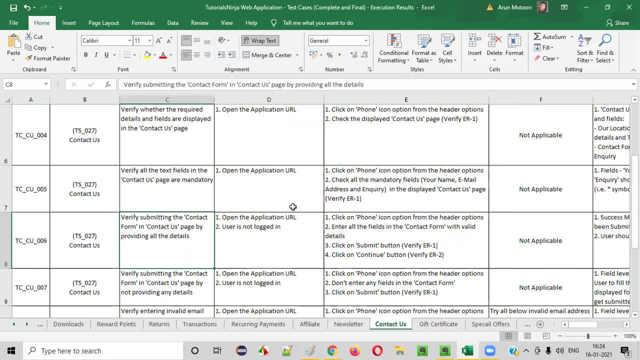 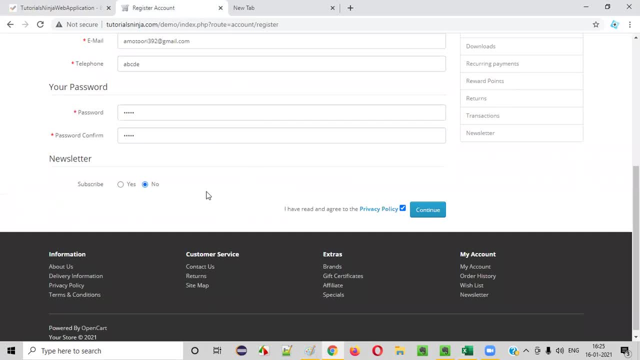 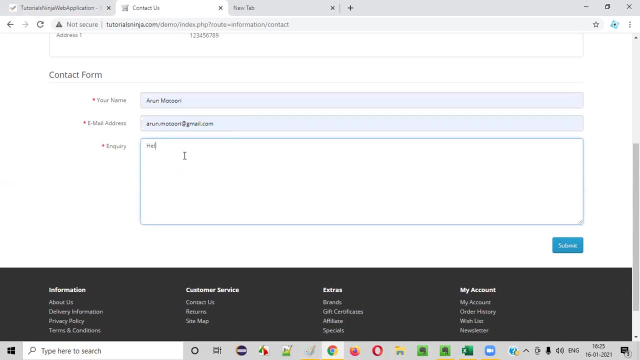 now we have to raise you to this particular test case to see whether the defect has really fixed or not by the developers. verify submitting the contact form in contact us page by providing all the details. so we'll go to the contact us page by providing all the details, okay. 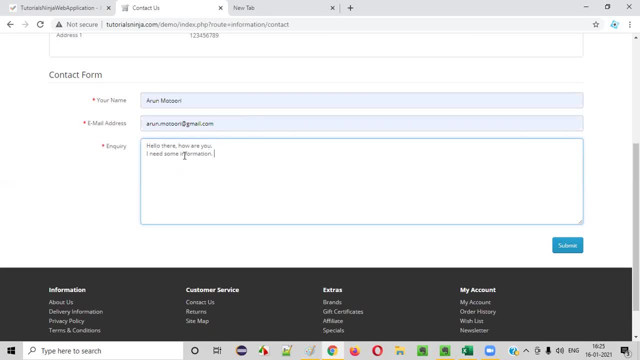 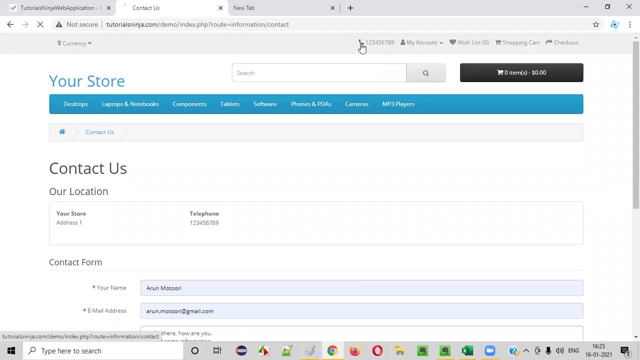 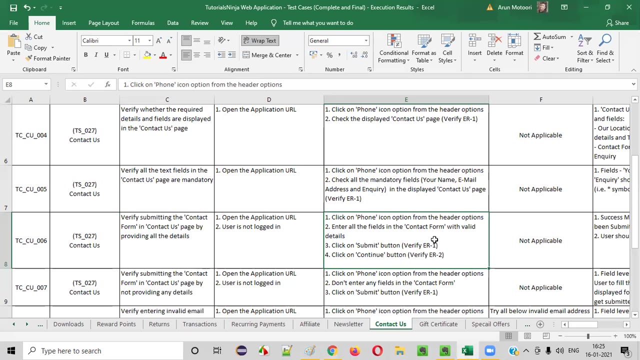 some dummy info. huh, i'm providing here and, uh, i click on the submit. right, that was the steps. right click on the phone icon. so you need to click on the phone icon like this so you'll be taken to the contacts page- contact us pay- yeah, contact us page and enter all the fields in the contact form. this. 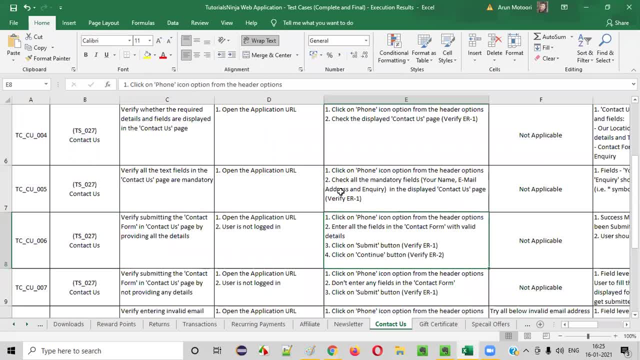 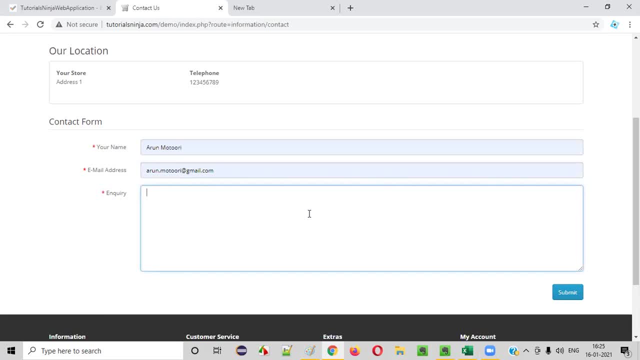 is the contact page form. guys, your name, email address and inquiry. you need to type, let's say, your name, you typed email address, you typed and okay, some message. you are writing. whatever it is okay, you want to message them as an inquiry, you can write it here and click on. next thing is click on the submit button. once you click on the 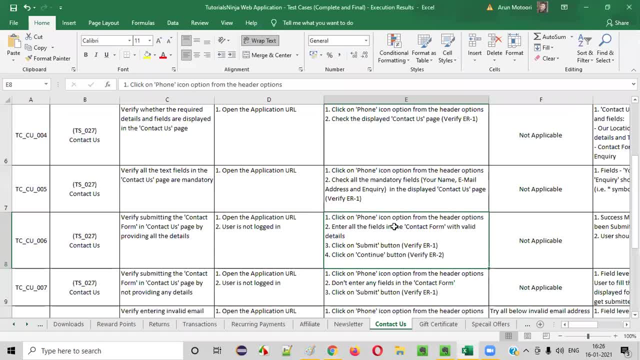 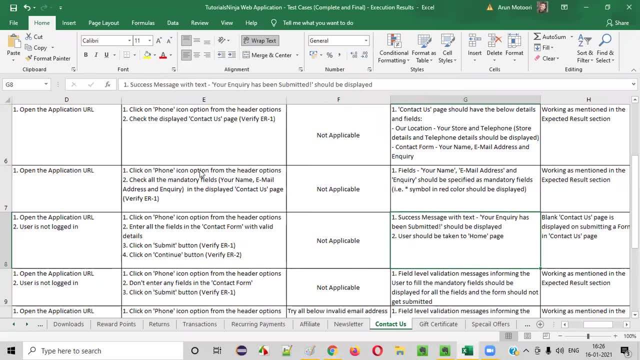 submit button. what happened, guys? some page is coming contact us pages. we have to verify this er1. let's verify the er1 success message with text. your inquiry has been submitted. are you getting any success message here? no success message is coming guys, instead what we are. 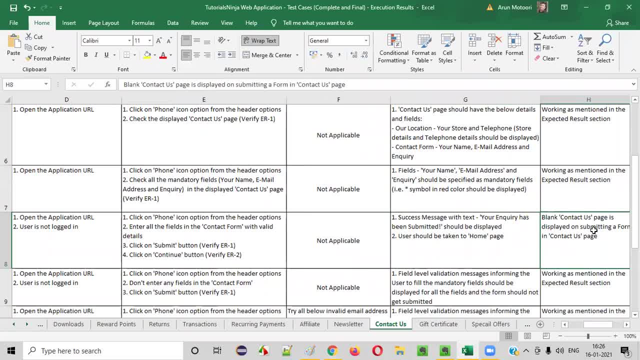 getting a blank page of contact us page is coming right. so here, whatever we faced in the version 1.0, still we are facing the same 2.0. also. you can write it here and click on. next thing is click on the submit button. once you click on the 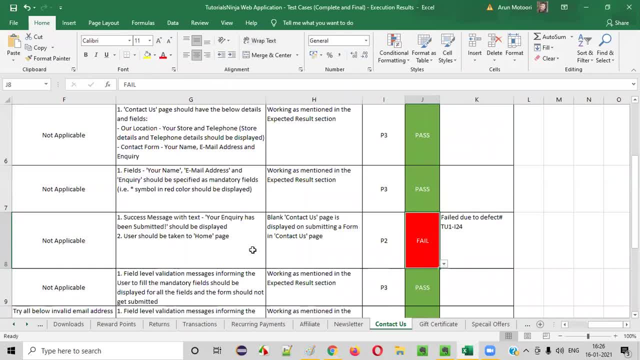 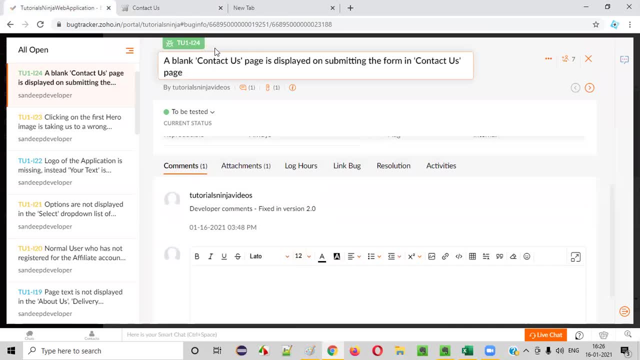 submit button. so what you will do, guys? okay, this will be still failure. only, this particular test case is still failing. only then you will go here and what you will do now? developers have mentioned that it, this particular defect, got fixed in version 2.0. but when you, when you have retested- 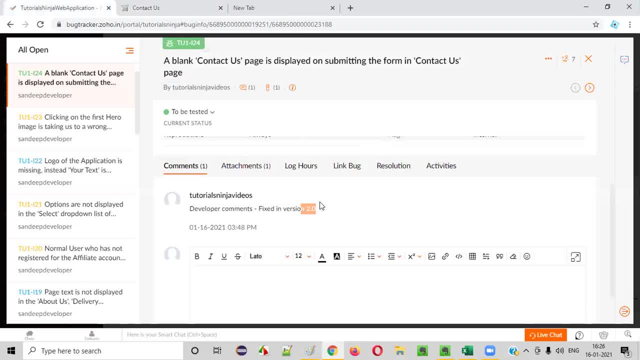 the test case related to this particular defect in this particular 2.0 version. the defect is still reproducing right, it's not fixed. actually, what you will do, guys, here, you will mention a comment saying that, saying that we have retested this defect in the latest version, 2.0, and observed that 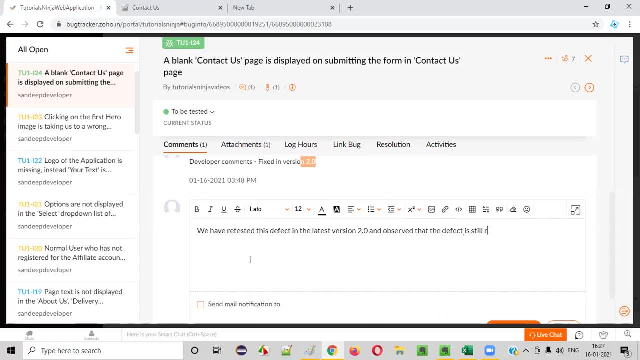 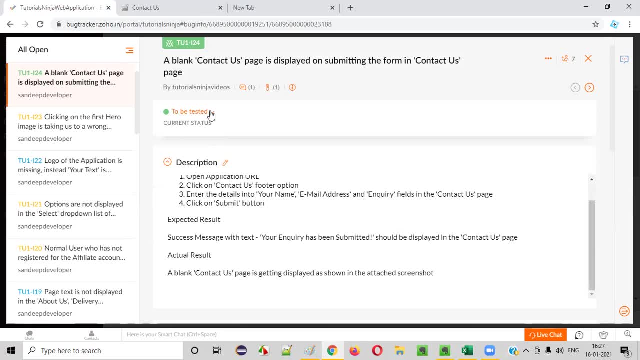 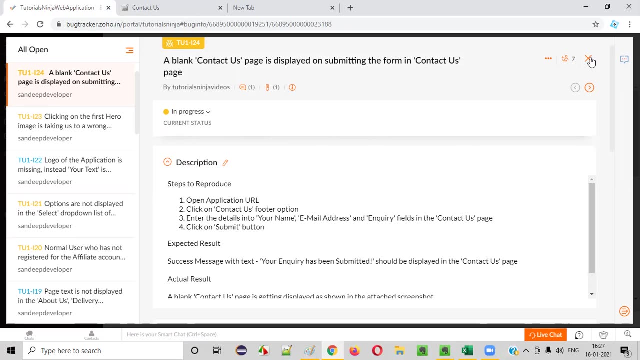 defect is still reproducing. okay, that means it is not fixed. so again, you have to change it to in progress so that it will be assigned back to the developers and developers will try to fix in the upcoming versions. so this is what we have to do, guys, as part of retesting, we need to 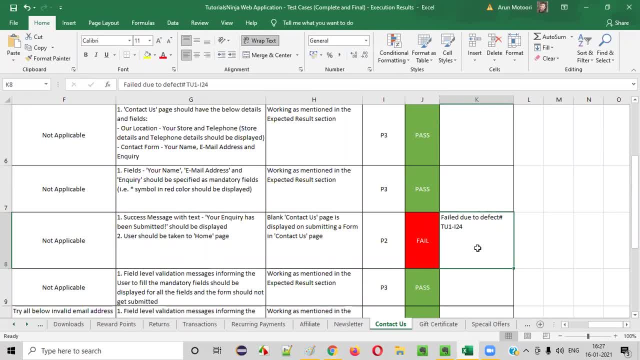 exude the test cases related to this particular defect with an intention of checking whether the defect is really fixed or not. all the test cases related to this particular defect need to be tested, guys. okay, that's what is retesting. hope you understood what is retesting now, right now, guys. 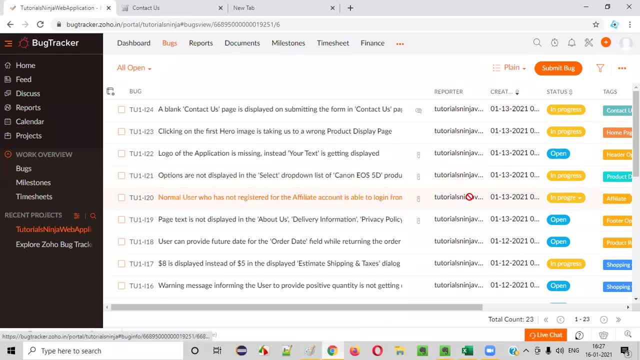 retesting is good. let's say uh here as part of this example, you have retested all the test cases related to the ready for testing kind of status defects, fixed defects. for all the fixed defects, you have retested the test cases related to the defect in the last version 2.0 and you can see that. 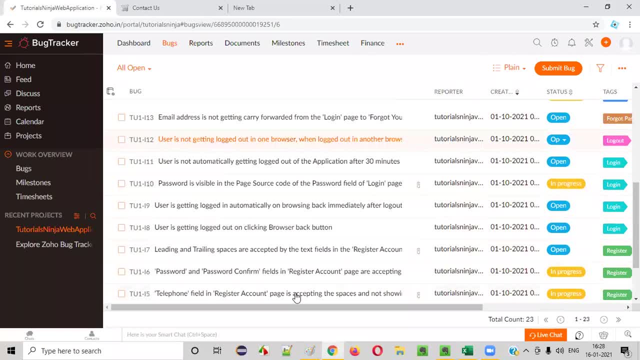 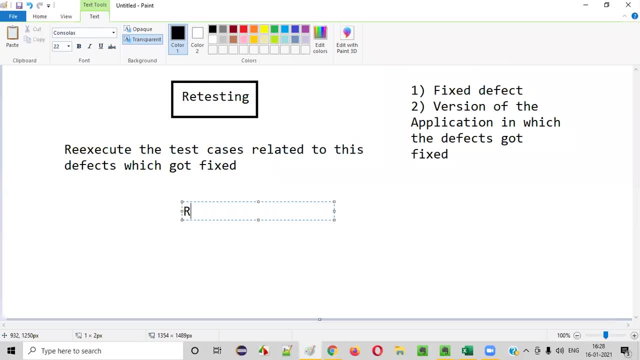 you have retested all the test cases related to the defect in the last version 2.0 and you can see that test cases we are as good as the risk cases, right, but guys will, retesting will be done. if retesting is done, then everything is done. no, guys, we have to perform one more thing, that is, regression testing. 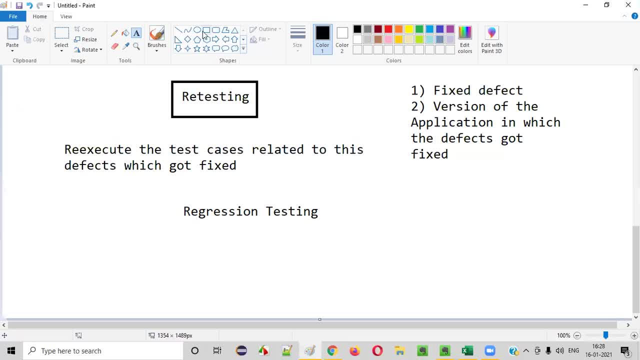 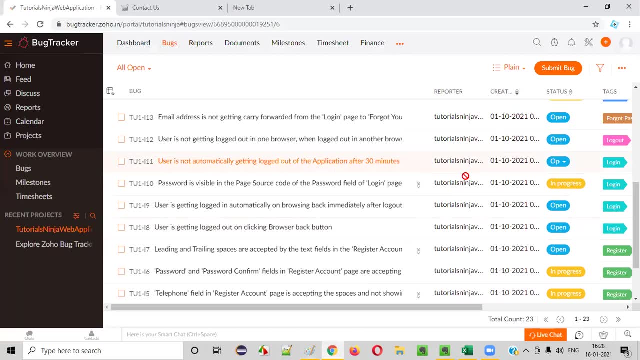 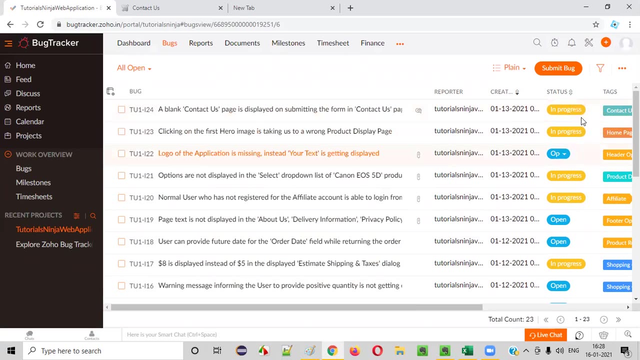 there is a reason why we have to perform regression testing. i'll explain. so what is regression testing actually? after performing, after completing the retesting, we are done with the retesting testing. right, we are done with the retesting because all that, all the defects which are, which were in ready, ready for testing state: right, we have retested them all. the test cases related to the fixed defects: we have retested them. right then, our task is done as part of retesting. now the next thing is, after doing this retesting part, we need to continue with the regression testing. okay, what is regression testing? regression testing means re-executing all the tester cases. okay, which? all the existing test cases re-executing? or, okay, re-executing all the existing test cases. here, as part of retesting, you only go to the test cases related to the fixed defects. 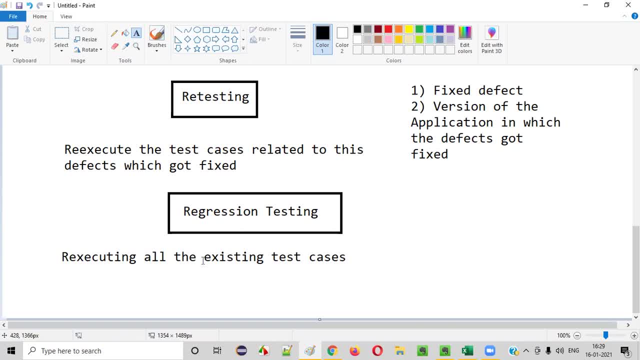 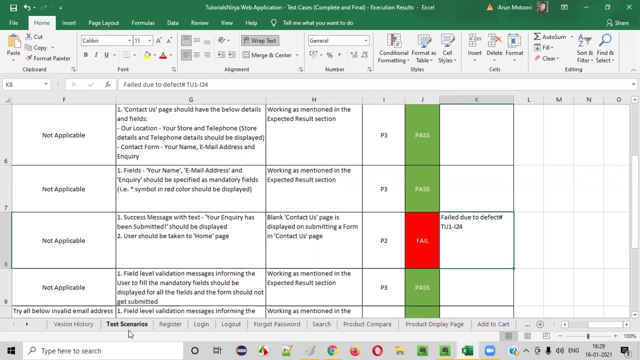 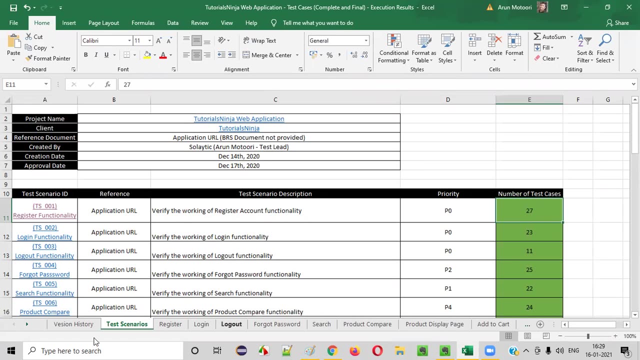 but here, as part of regression testing, you are re-executing all the existing test cases. that means starting from the beginning. guys, you have to execute. okay, so these are the test cases. right for register functionality. how many test cases are there? 27 test. you have to again execute the 27 as. 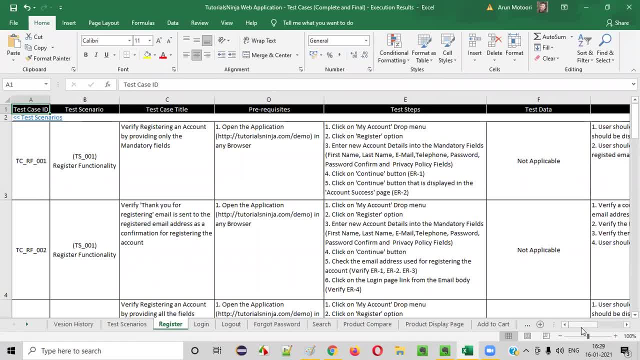 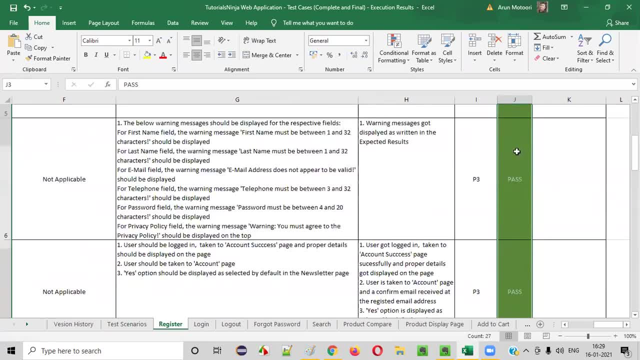 part of the the first cycle, you executed all these test cases and updated with the results right here. you see in your in the first time you executed all the test case and you have provided the results here properly: right: pass for pass, fail, fail, file pass and all those stuff. okay, like that you. completed all the test cases already. but again, guys, when you get a latest version with some defect fixes right, then again you need to retest. i mean, again you need to perform regression testing, where you need to exclude all the existing test cases. so why we need to execute all the test cases? right. what is the logic behind this, why we have to perform regression testing? so till now i didn't give a proper definition for regression testing. guys, i am able to give, but for now you need to understand this logic. so when a developer fixed some defects and gave you the latest version in which this particular defects got fixed, you can simply re-execute the test cases for which the effects got failed right earlier. right, only those test cases will be enough. but here, as part of regression testing, i am insisting you to perform regression testing, where you need to execute all the test cases, not only the test. cases for the defects which were fixed, but also you need to execute all the existing test cases. why i am saying that? why regression testing will say that you have to re-execute all the existing test cases thing. here is: guys, this is a logic. okay, let's say: this is application. the application has 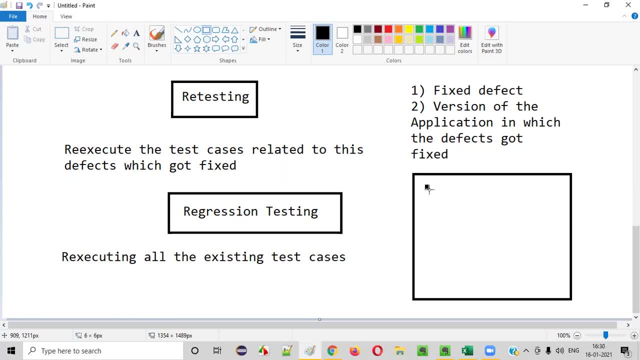 a lot of functionalities. let's say you have reported a defect for one of the functionality. okay, you have reported a defect, for there is a problem in this particular functionality and you have reported a defect for this. now the developers have said that we have fixed this particular. 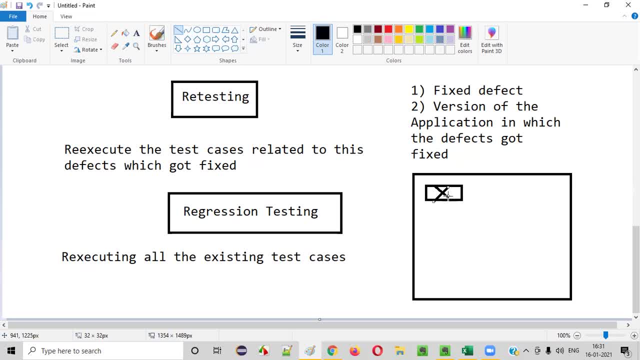 defect, only this particular functionality. they have modified the code and they have fixed the defects. now, as part of retesting, you as go to the test cases for this particular defect. right, whatever the test case related to this particular defect, you have re-executed and somehow let's. 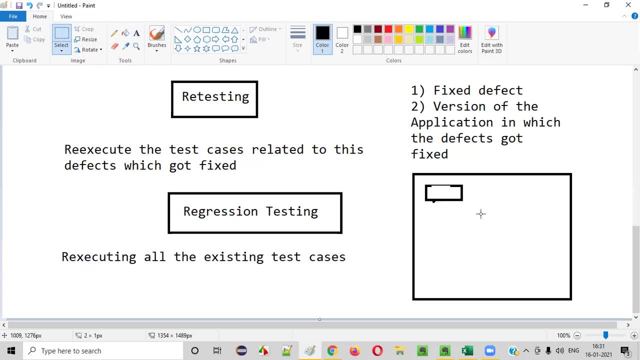 assume that the defects are passed. okay, they got fixed successfully. you have closed the defects. you have simply closed the defects. let's say like this: now, after retesting is done, you have to perform regression testing. that means you have to check the all the other existing functionalities of the application, not only the functionality for which the defect got fixed. you need to test, but also you need to retest. i mean, you need to re-execute all the existing test cases for the remaining functionalities. why so? why, guys? what is the? what is the reason here? this functionality tested will be fine. right, all the test cases related to this defect related. functionality will be fine. but here we need to test the existing functionalities, all the existing functionalities for which the test cases were already created right, just because of this particular fixing of the defect, i need to test all the remaining functionalities also. why? why, as part of regression testing, i need to check each and every functionality of the application. 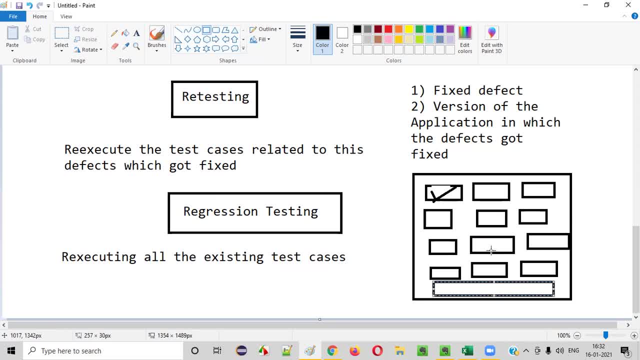 not only the functionality for with the defect got fixed, but also the other remaining functionalities of the application also needs to be checked, okay. so the reason here is: whenever a developer fixes, okay, this is the reason. clearly observe guys, clearly focus on this why we perform regression testing. you need to understand. clearly. okay, that's why i'm insisting so. so why we need to perform regression testing, that is, executing all the test cases of the existing application, our functionalities of this application is the. the reason here is the main reason here- is when a developer fixes this particular defect in one of the functionality, there may be at least a test case of the existing. 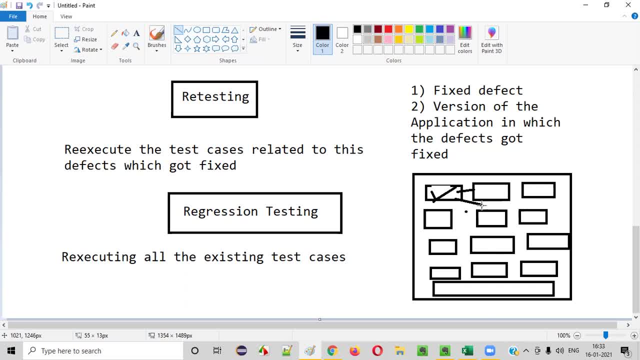 may be a chance that other functionalities may get affected. okay, because of this particular fix. okay, there may be some side effects. okay, in the other functionalities of the application. as a tester, we cannot take it for granted, guys. okay, so we have to test each and every. because of this. 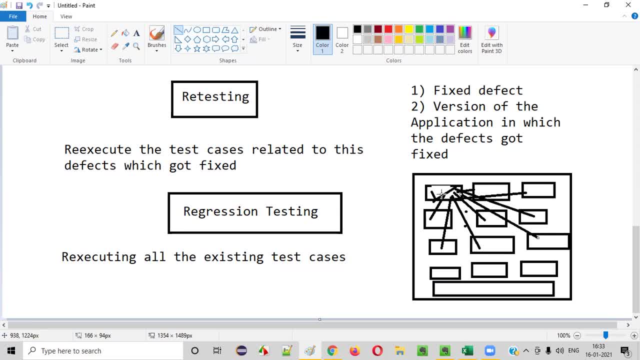 particular fix in this particular area of the application. this particular fix may introduce some new problems in the existing areas of the application. we don't know right, because it is at the core level, it's not at the ui level. you may think at the ui level and see that everything is. 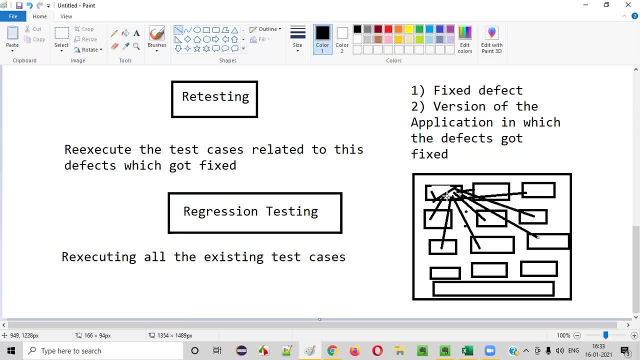 fine in this particular fixed section, but internally the code may get disturbed- we don't know what will happen inside the code as a tester- and it may result in some new defects in the existing working functionalities of the application in the previous. let's say because of the existing working functionalities of the application in the previous, let's say because of. 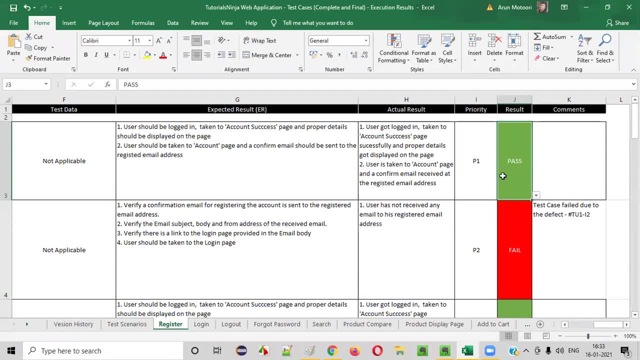 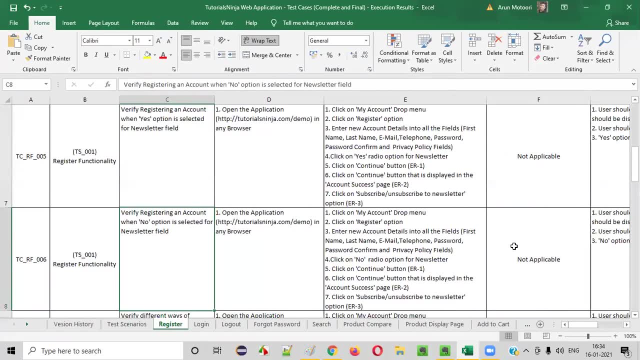 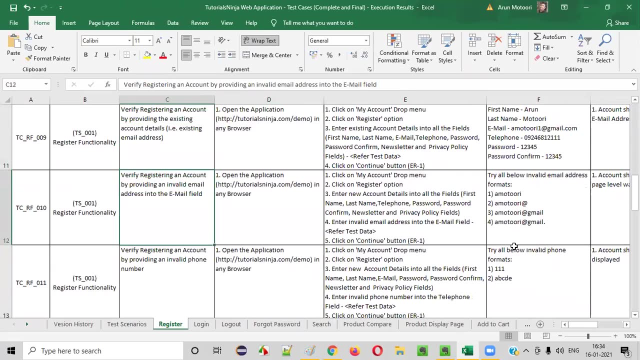 this particular fixing of the defect. let's say, one of the defects got fixed right. uh, what was the defect, guys? so let's see the defect. uh, phone number thing- right, where was the phone number? yeah, this was the one. let's say, this particular defect got fixed, right we. 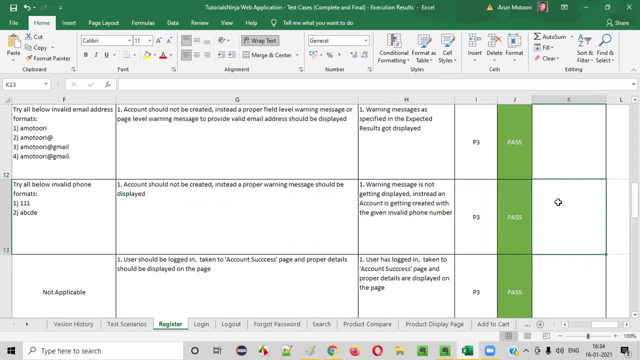 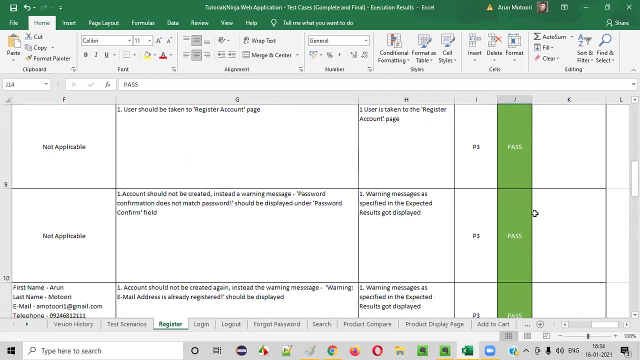 we changed it to pass right this. there was a defect here and this got fixed and it got passed. and because of this particular fix, in this particular defect, this defect may okay, because of this particular fix, the next test case may also get failed, we don't know what. okay, some some other test cases may fail earlier. these test cases were passing. 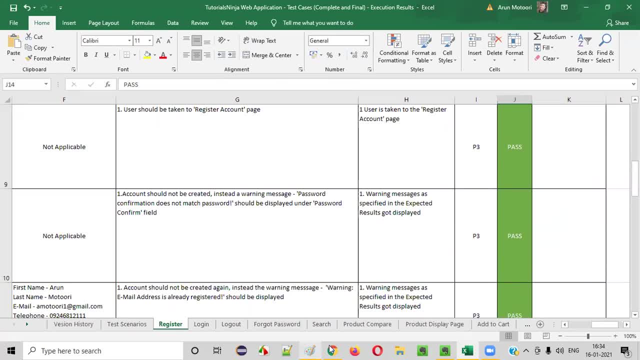 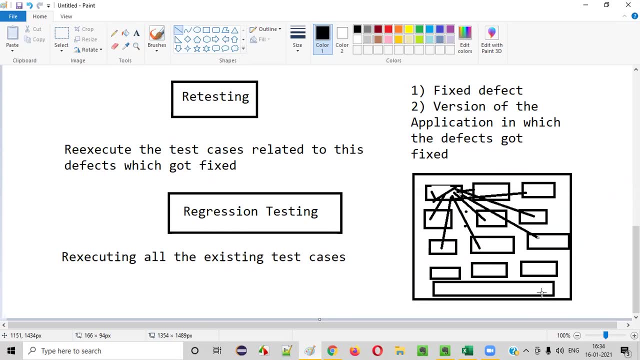 now, because after the fix, some test cases may fail. this is all because, because simple reason guys: side effects. okay, defect fixing may have side effects on existing working functionalities of the application. the earlier working functionalities may get affected because of this fixes, defect fixes. so not only defect fixes, guys. if a new functionality, tomorrow a new, 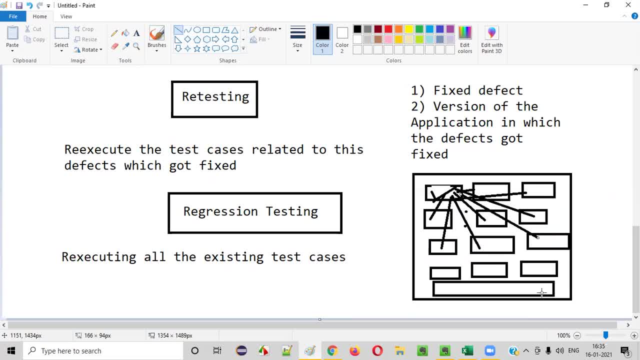 functionality is added to the application. now, let's say, there is only one payment gateway, right, cash on delivery- in our application. as you already know in the previous sessions now tomorrow, the like developers have written a new code where they added another functionality, like where you can do credit card payments also. let's say, okay now, because of that new functionality also existing. 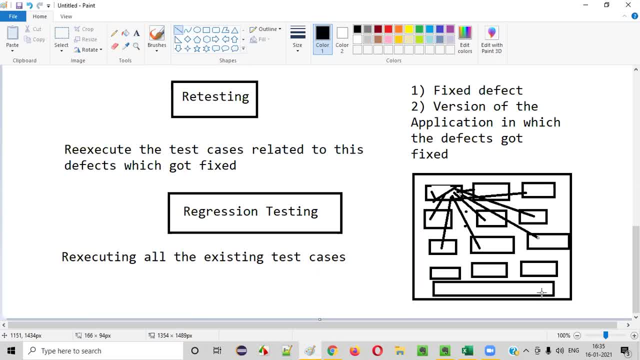 code may get affected. there may be side effects. generally, regression testing is performed when, like when there are some defect fixes and also when there are some new functionalities introduced into the application. because of that, code changes will happen. that code changes may reflect in some side effects in the 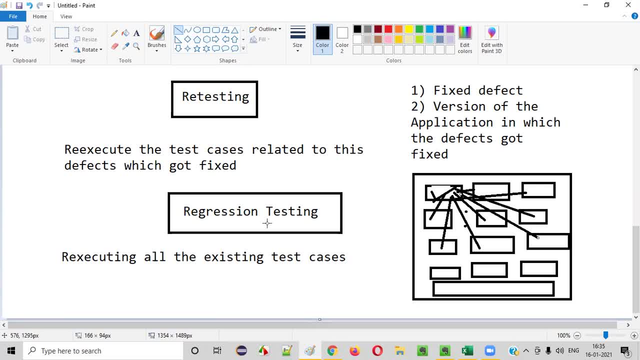 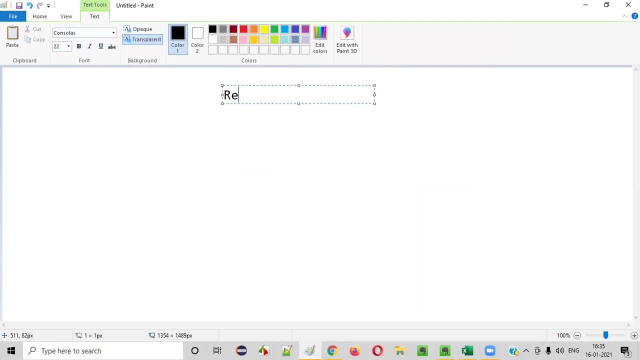 existing working functionalities of the application. so this is the reason, guys, we have to re-execute all the existing test cases as part of the regression testing. so, no matter what, okay. so these are the two things, guys. okay, what you have to do. just let's revise again so that it will be more clear for you guys. 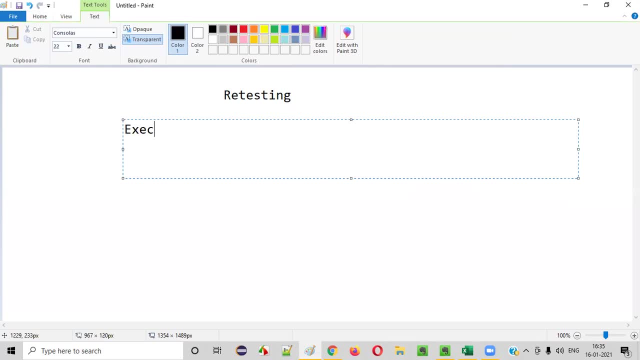 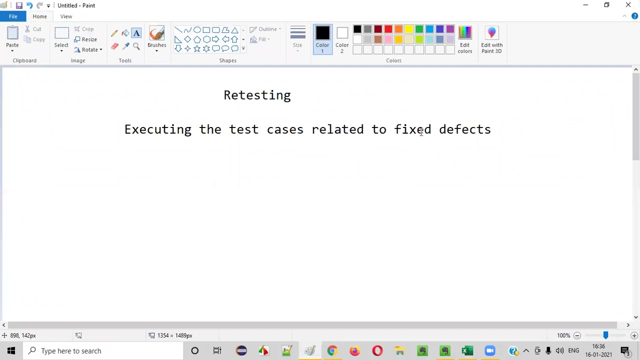 first thing is retesting right. retesting means what guys executing the test cases for the fixed defects? test cases related to fixed defects earlier. whatever the test cases, you have failed and reported the defects right. that particular test cases only. you need to retest as part of retesting to check whether 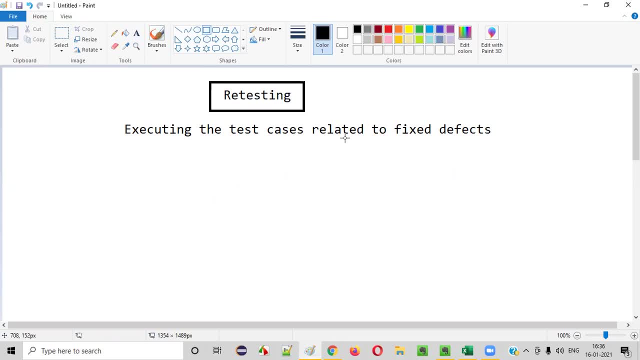 the defects are really fixed or not, you need to re-execute the test cases which have led you to report these defects. that is the one thing. next thing so, because of this- defects fixing happening after the defects got fixed- the code level changes may happen and which may actually introduce some side effects into the existing. 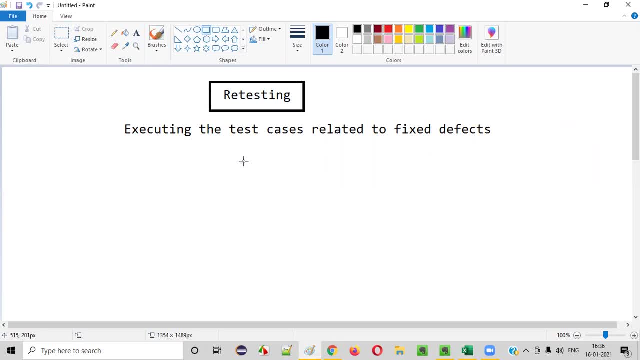 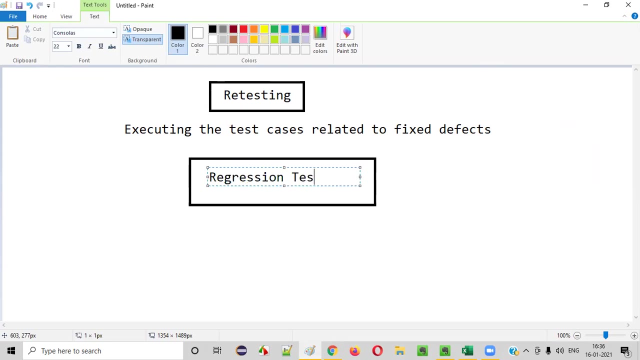 functionalities of the application which were working fine earlier. to overcome that, to check whether the existing functionalities are not affected by this change. okay, because of this fixing of the defects, the existing working functionalities are still working as expected or not. for that, what we have to do, we have to perform regression testing. how to perform. 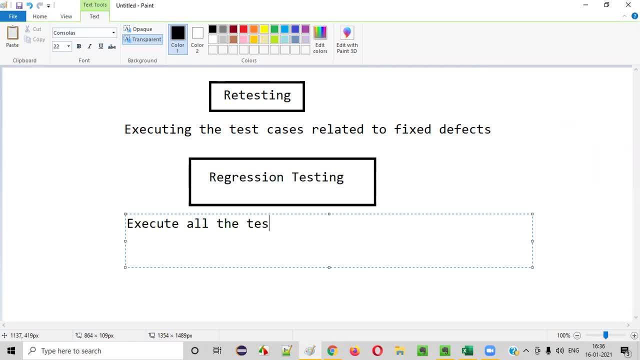 regression testing. we have to execute all the test cases. all the existing test cases, guys, no matter what. okay, all the execute existing test cases, irrespective of whether they are working fine or not, it doesn't matter. all the existing functionality application test cases need to be tested from starting to the end. that means this complete test case document need to be. 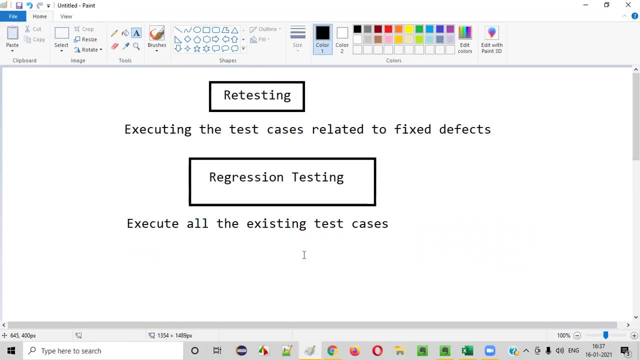 executed again as part of the regression testing to see whether there are no side effects in the application. because of this fixed, because of this defect fixes, there are no side effects in the existing functionalities of the application. that is regression testing, guys. so another situation where you need to perform regression testing, apart from the defect fixes, is that 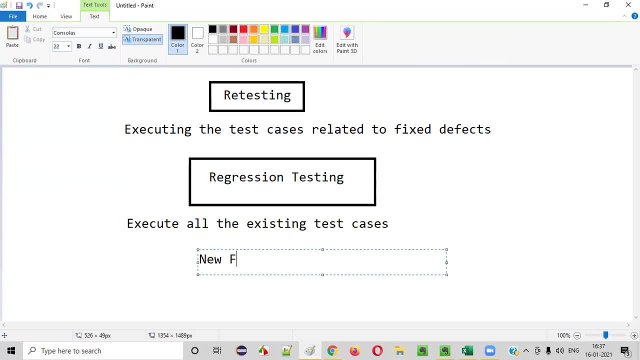 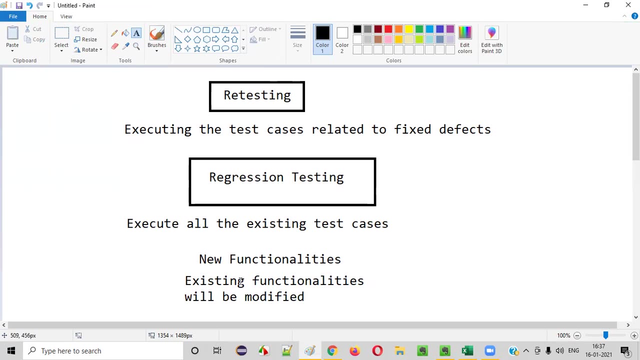 where sometimes in the application new functionalities will be introduced or some existing functionalities will be modified. existing functionalities will be modified, okay, just to uh, some requirement changes will happen and some existing functionalities are modified, some defect fixes may happen, some new, new, latest functionalities may get added to the application. whatever it is, guys, whatever the code, changes happen every time. 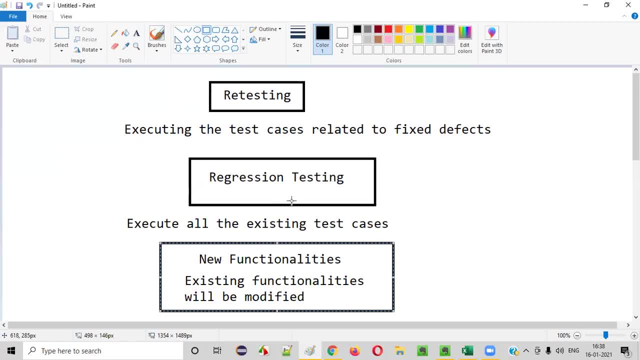 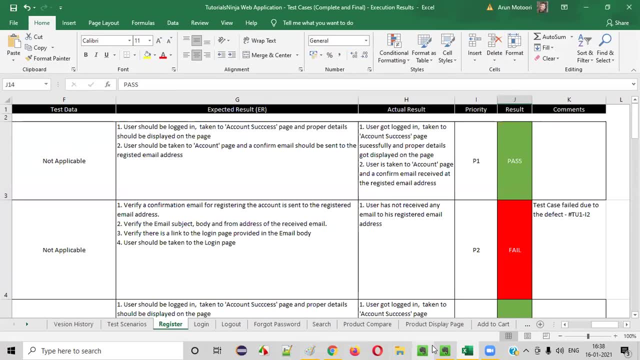 we need to perform regression testing to see that there are no side effects in the existing working functionalities of the application. so hope you understood, guys. so what next guys? so as part of these uh, retesting and regression testing, we have to execute the all the test cases: failed test. 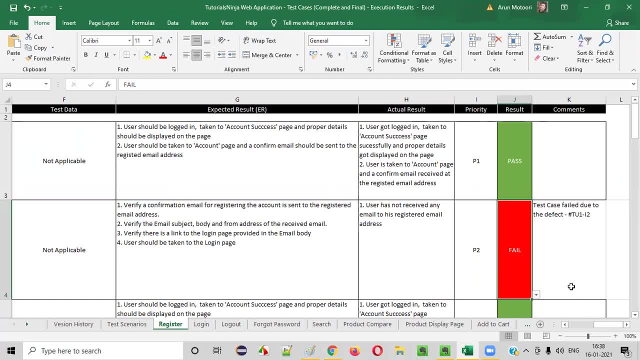 cases for which the defects got failed. is retesting all the test cases to see whether they have any side effects or not. is regression testing okay? so don't think that we'll execute the test cases only once. in testing there are multiple cycles, guys. we generally call them as testing cycles. 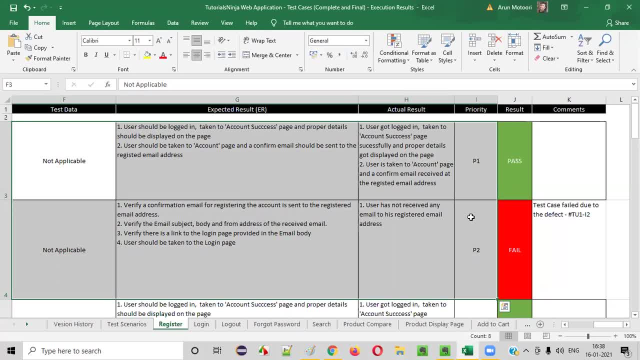 the moment you get a new version of the application, as a duty, as a duty of the testers, we need to perform you to see whether the test cases related to the defects got fixed or not, i mean, are working fine or not okay. and second thing is to see whether there are no side effects in the existing working. 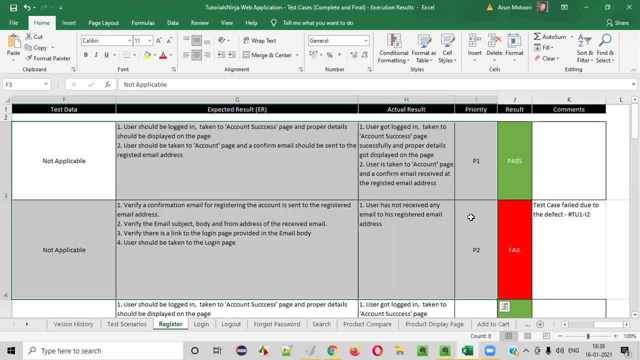 functionalities of the application, where we need to execute all the test cases, all the existing test cases of the working test cases. whatever it is, we have to test it completely. so, so, so what we have to do is we have to test this complete test cases, from register functionality to the all the test. 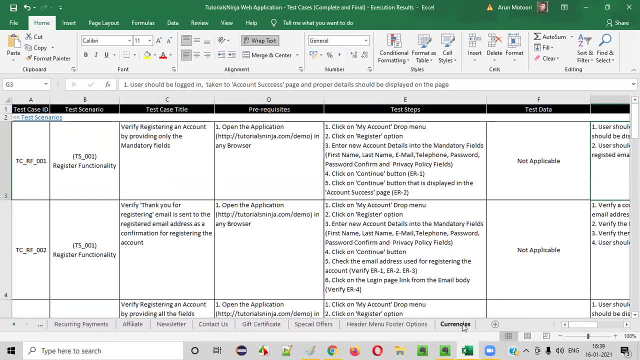 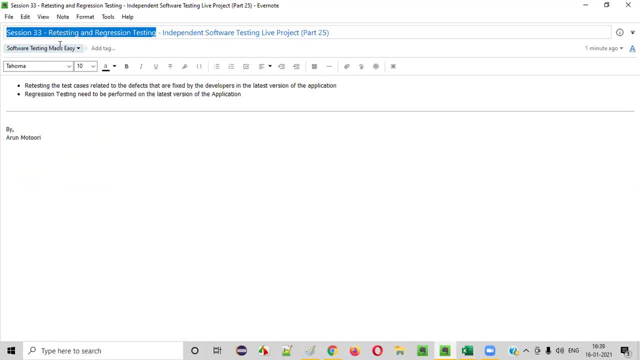 cases in this part, all the tabs we need to test again in the latest version of the software. so we have to do this in the software, okay, so hope guys, you understood what we do as part of retesting and regression testing, right, so what you have to do next after you are done with retesting and 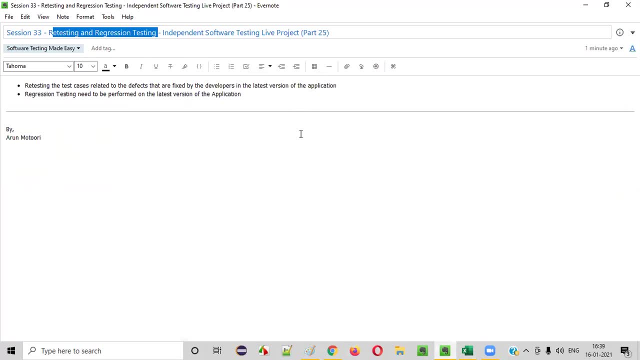 regression testing in the latest version, that is, let's say, latest version is 2.0. right, let's say you completed retesting and regression testing. what? what you will do? you have to send an email to the client guys status email to the client. by this time you perform this retesting and